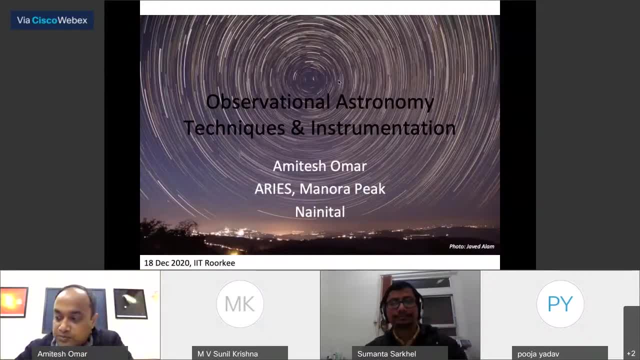 Sir, the live streaming is on now. Okay, Good evening to you all On behalf of the. Good evening to you all On behalf of the Indian Physics Association Rurki Chapter and Physics and Astronomy Club and Department of Physics IIT Rurki. 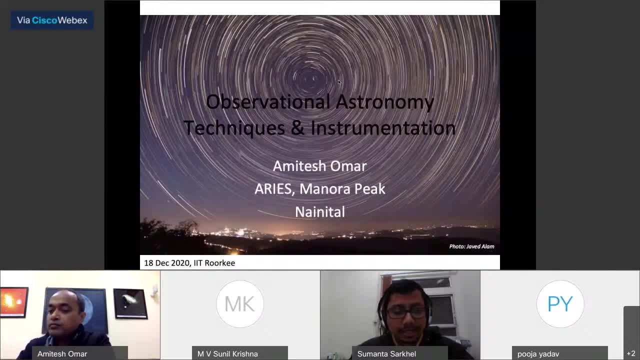 I welcome you in this lecture series: Astro with Aries. So this is the third talk in this lecture series and will be delivered by Dr Amitesh Omar. So now I request my colleague, Professor Sunil Krishna, to introduce the speaker. Hello everyone. 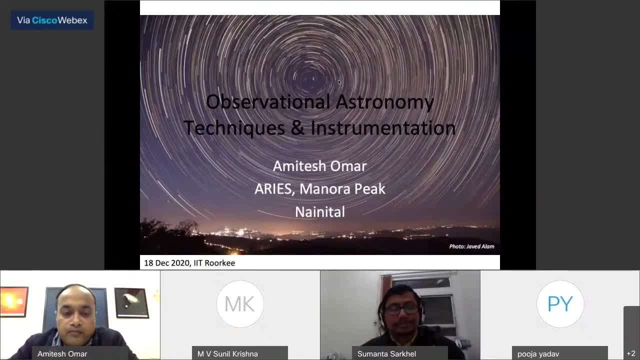 Good evening to all. So I am glad to introduce Dr Amitesh Omar, who is today's speaker. So Dr Amitesh Omar is an astrophysicist working in the area of galaxy evolution and optical instrumentation, with experience in both radio and optical astronomy. 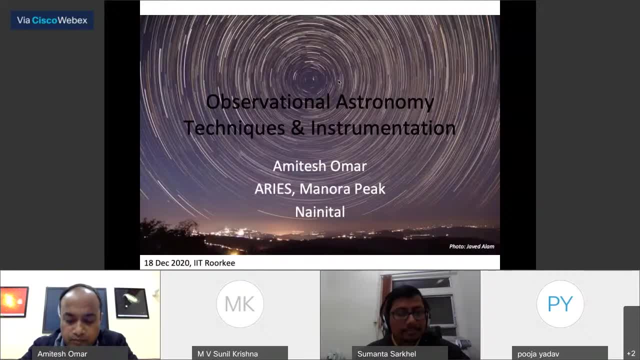 He completed his PhD from Ramanujan Institute, Bangalore in the year 2004 and his MSc was from IIT Delhi in 1997.. He was a post-doctoral fellow at Leiden Observatory in the Netherlands, working on the design aspects of. 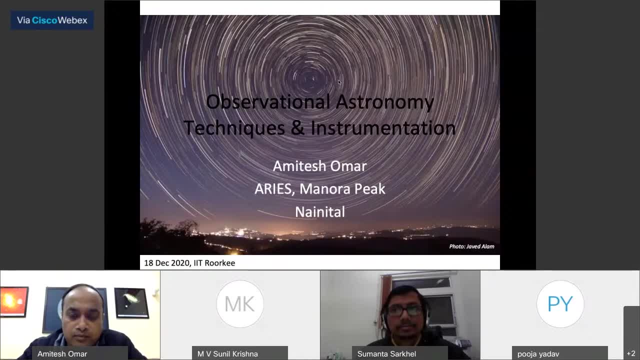 low-frequency radio telescope arrays. He was part of the team To establish two observable facilities in the 1.3-meter and 3.6-meter optical telescopes in Devasthal Observatory in Uttarakhand. Recently, an optical spectrograph has also 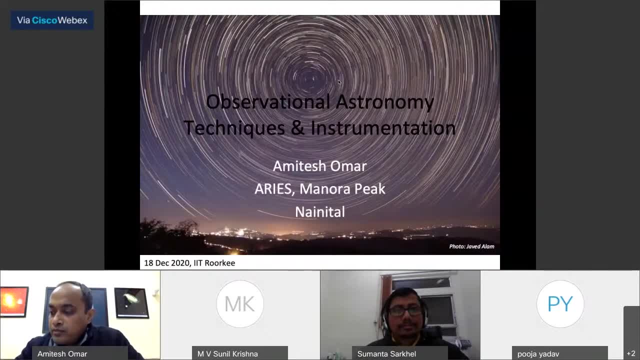 been commissioned on the 3.6-meter Devasthal optical telescope. Through this in-country design and development efforts under his supervision, he is leading this research. So with this brief introduction, I request Professor Amitesh Omar to kindly deliver his talk. 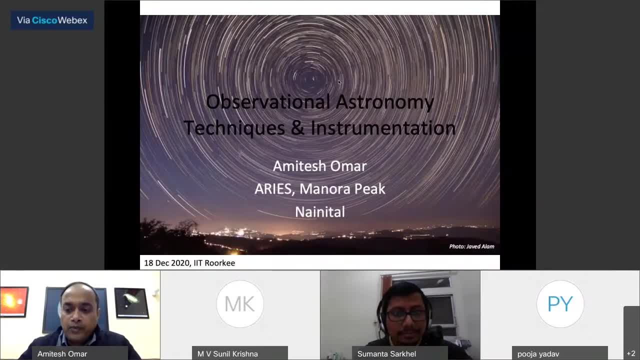 Thank you, Professor Sunil. Yeah, thank you, So I can start now. Yeah, yes, please, OK, So welcome all. I will be taking you through some aspects of observational astronomy, particularly the techniques and the instrumentation. Now, of course, we 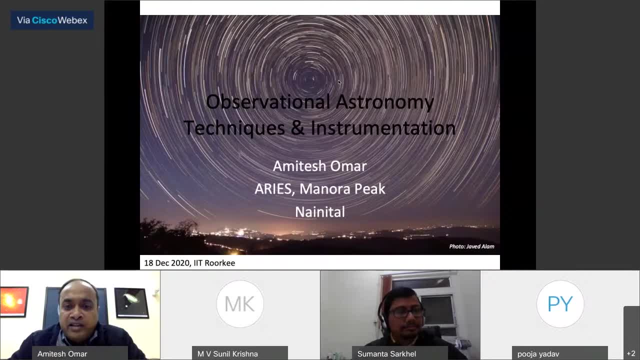 All you know take interest in astronomy either as an amateur or as a professional, And so we are familiar with most of the things in the sky, like stars, And some of you might have seen galaxies, And some of you who go a little bit advanced. 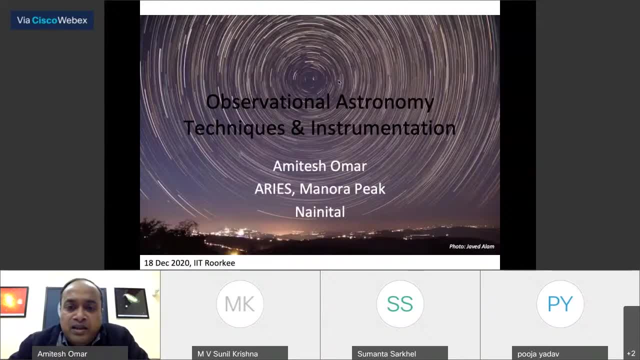 might have also made some images. I'm sure Every National Institute now has a major astronomy club, And I see that IIT Roorkee also has such a club there, And I'm sure that they must be doing similar things. Let me just see if this works. 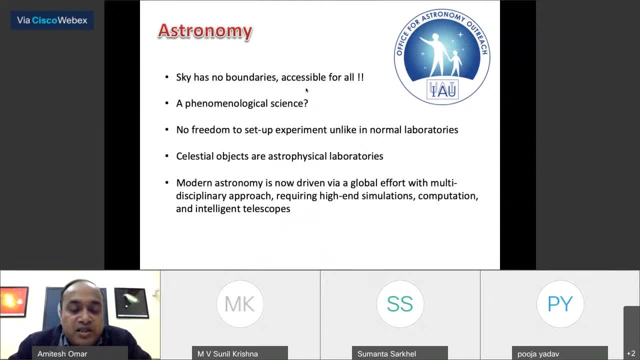 So astronomy, of course, as we know, has no boundaries. This is accessible for all, And that is what this logo of the International Astronomical Union tried to say: that it has no boundaries open for all. Most of astronomy has been work as a phenomenological science. 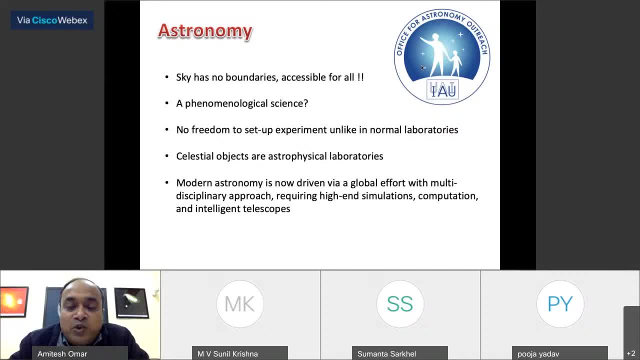 what we call it, And that means it's based mostly on phenomena, what we see, Because we do not have a freedom, unlike if you work in a lab. we do not have a freedom to set up experiment And whatever is given to us, we actually observe that. 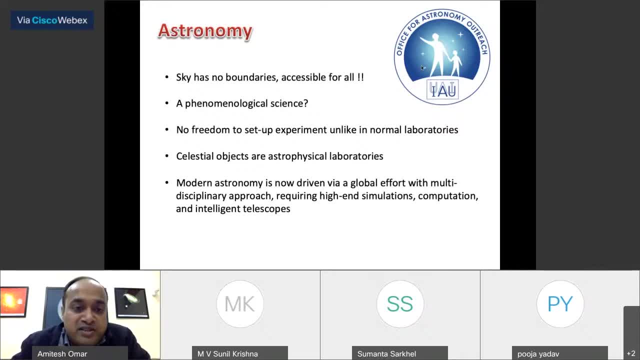 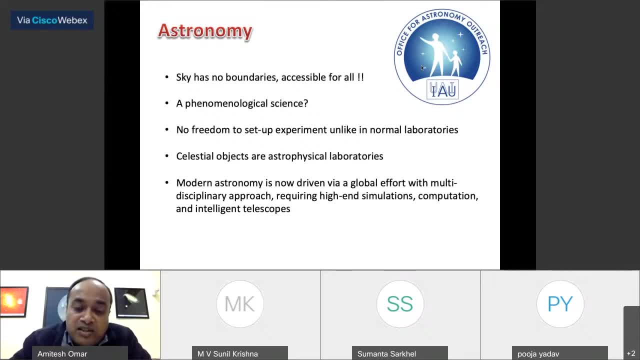 is driven by a global effort with multi-disciplinary approach. It requires high-end simulations, It requires very high-end computation, as well as the telescopes which are intelligent. So if you remember the earlier telescopes where one has to go and look at that, you know through the eyes. now that's no longer there. we have sophisticated. 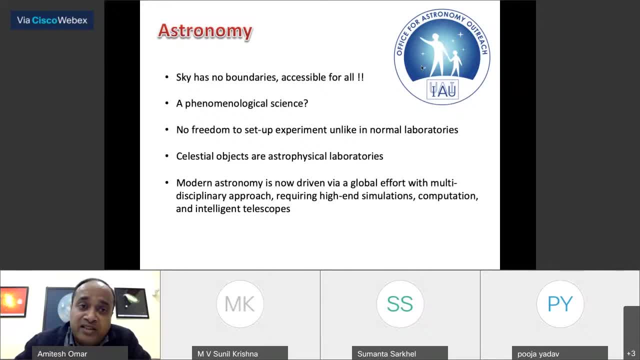 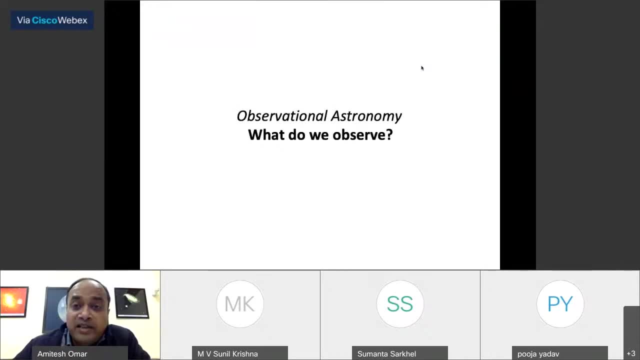 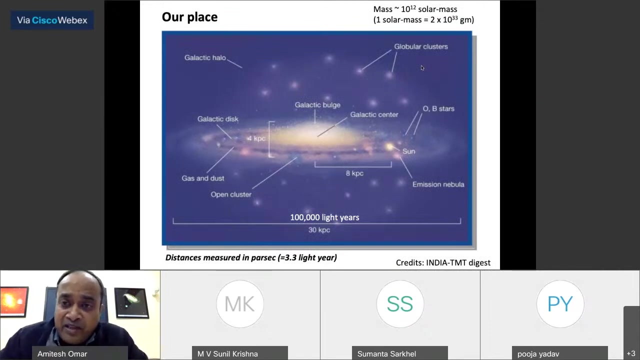 cameras and the telescope themselves are quite intelligent. they can sort of learn what to do over the time. let me first take you to the observational astronomy. what do we actually observe? and this will be a very brief introduction for beginners, and i'm sure most of you at an advanced level might have seen. 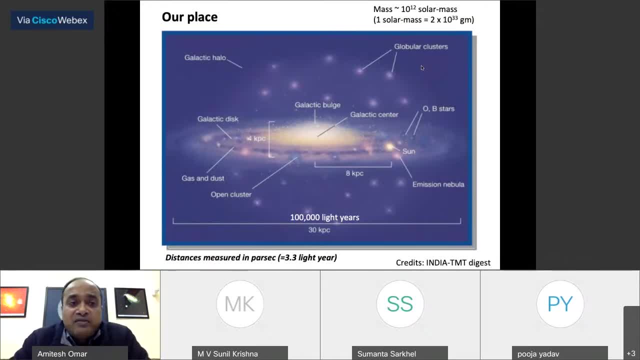 or you know such pictures. so let me start with our place in the universe or our place in the galaxy. let's see what we see. here is the image you know a, a cartoon image. it's not a real image to see of how our galaxy looks like and what are the different components of our galaxy. 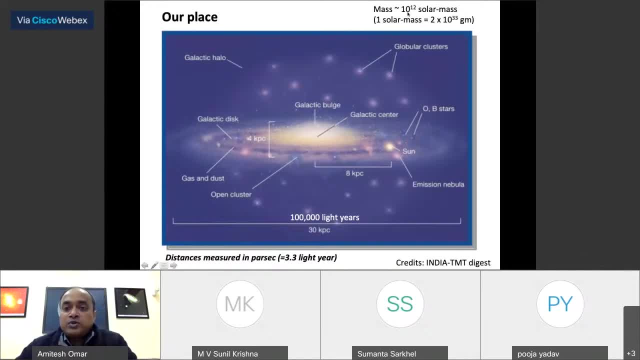 our galaxy has a huge mass. first thing, that's about 10 to power, 12, 12 solar mass, and you know that one solar mass, what we say, is the mass of our sun, which is approximately 10 to power, 33 grams. what you see in this picture is that this is 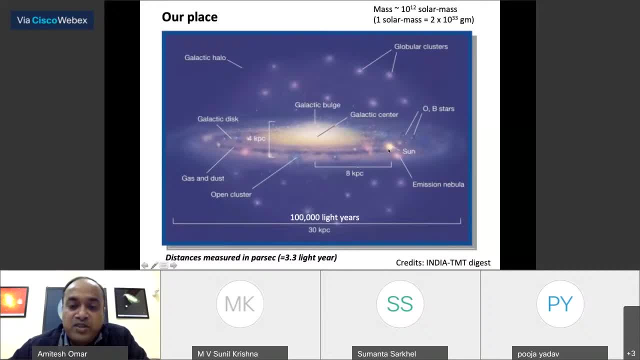 the disc galaxy and sun is here, which is roughly 8, 8 to 10 kilo parsec away. so we astronomers measure distances in parsec, which is equal to 3.3 light years, and so whole galaxy, our milky way, is of the order of 100 000 light years. we have lots of structures in this, what we call the 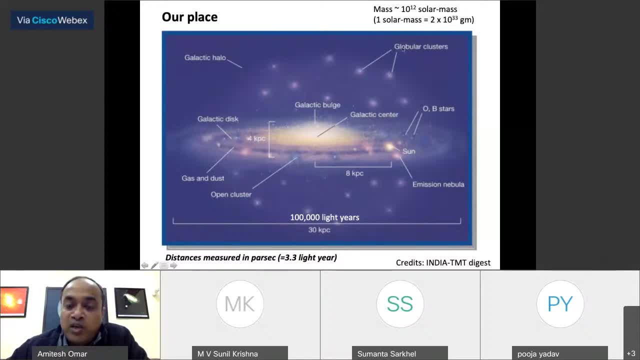 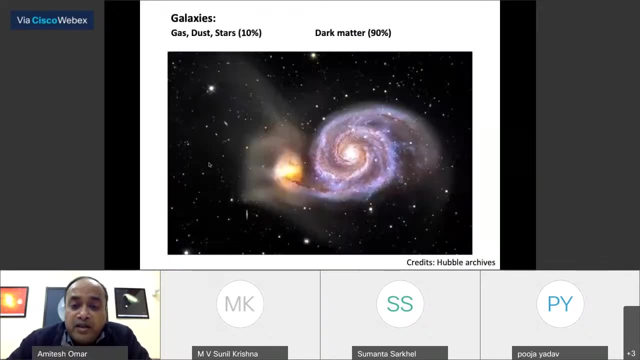 galactic disc, we call the galactic halo, which has one of the oldest object in the universe, which are known as globular clusters and very young stars, nebula clusters, gas and dust, in fact, now of course we have. we cannot image our own galaxy, but we can actually look at. 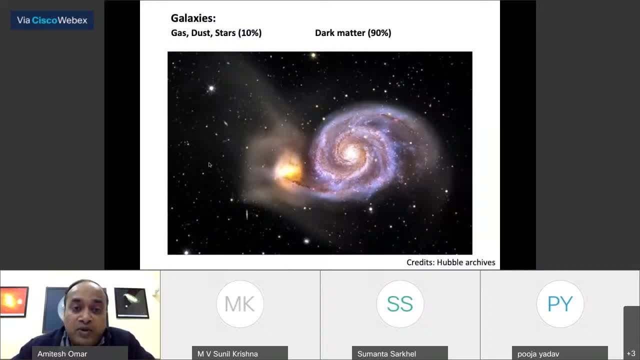 other galaxies which are very similar to our galaxy, our milky way, and we know a lot about such galaxies and what we see here is a very, you know, catchy, eye-catching picture, very beautiful picture, which hubble space telescope keeps on taking, and what we know scientifically is that our galaxy as well as other galaxies, so our galaxy is not as 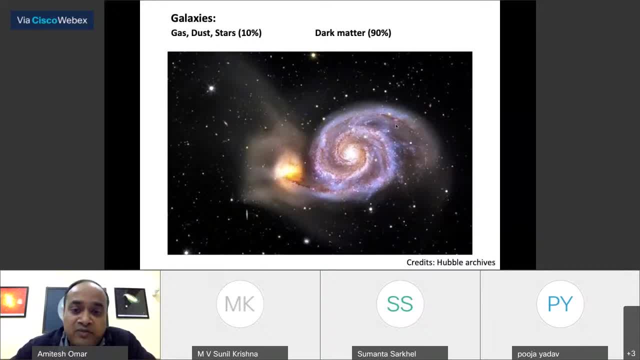 special galaxy. it's a very similar to other. you know billions of galaxies present in the universe. this consists- the gas dust in stars which we can observe directly is only about 10, and this, of the material, is 90, is the dark matter for which we really do not have much understanding. 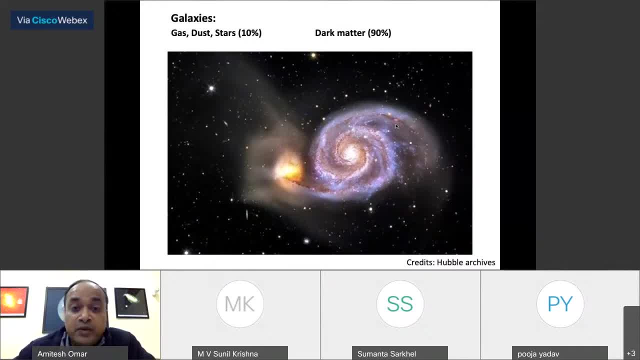 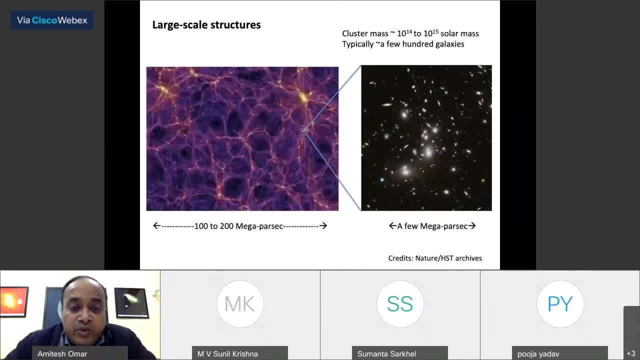 but we know it from the dynamics of galaxies that there is a gravitational force related to the dark matter, the scale structures in the universe. it looks like a very spongy kind of feature: lots of places where there is nothing happening. there are some places where lots of things are happening. so what is? 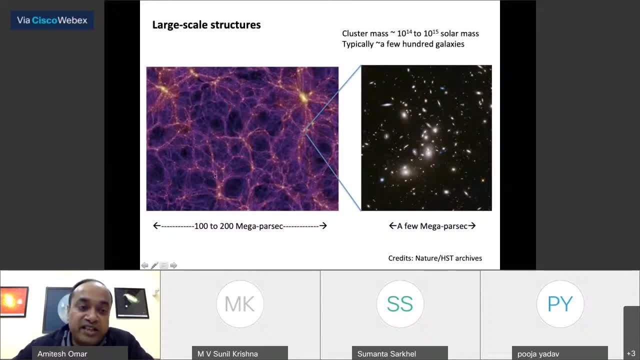 shown here is the dark matter distribution, or we can actually trace the galaxies here. so all the bright points here are representing clusters of galaxies, which is one of the typical cluster of galaxies shown here. again, taken from havali space telescope cluster, can have very large mass. in fact these are the largest boundary structures in the universe gravitationally. 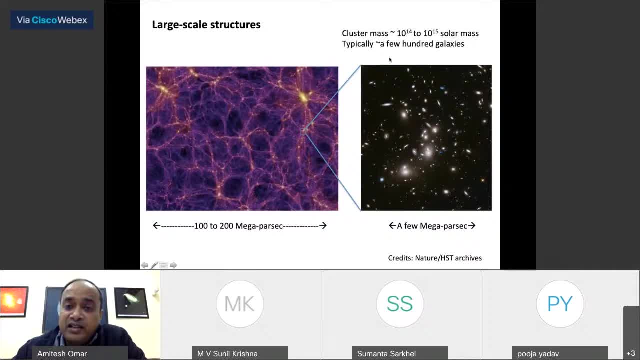 bound structures in the universe. any cluster can contain typically a few hundred galaxies and that's about a megaparsec. you know the size, and what you see here is of the order of about 100 to 200 megaparsec structure and that structure is present all over the in all the directions. 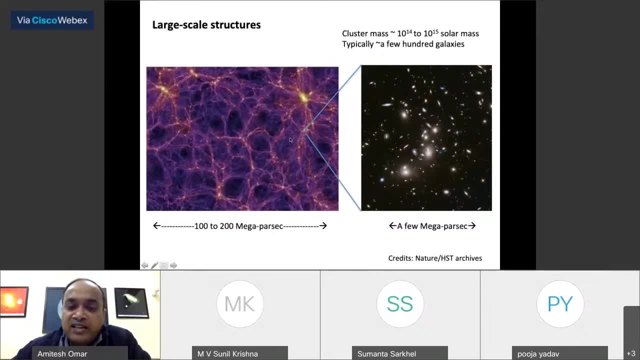 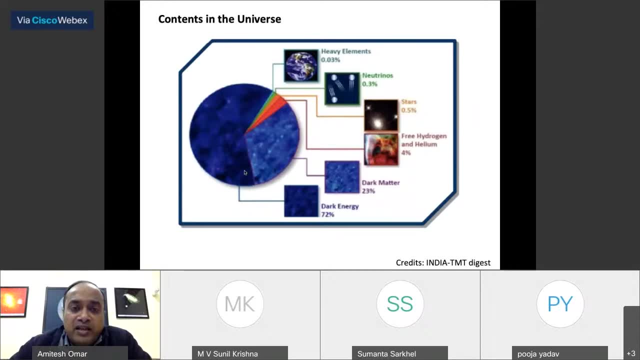 you know which we look at. we actually see this larger scale structure. now this gives rise to a estimate, basically a budget of the universe, what universe is made of. so, if you look at this, there are heavy elements which are made of about 0.03 percent. we all are. 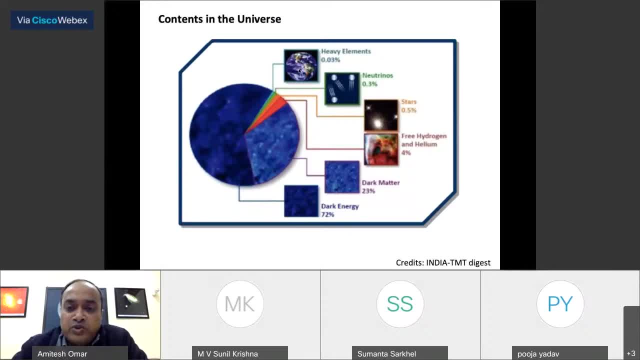 made of heavy elements. then there is there are neutrinos, which have a small fraction- it starts only about half percent- and the universe is filled with mostly hydrogen and helium, which is about 4- and then, of course, the dark matter and the mysterious dark energy. the point to see here is that what we observe here is a very small fraction, typically, of the 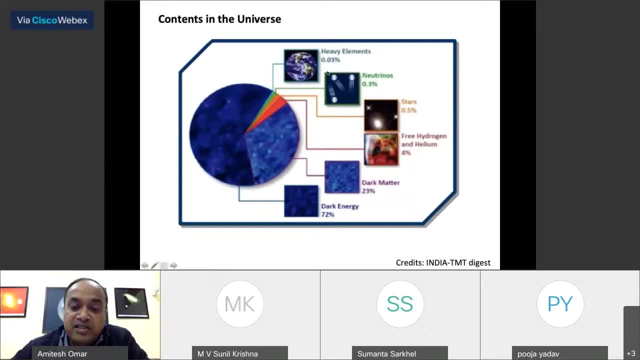 order of five percent. what we can actually observe and rest is not observable by any known technique so far. so we actually look at very small fractions, for example, stars. if you look at what we look at through the optical telescope, It's only a very small fraction by mass of the entire universe. 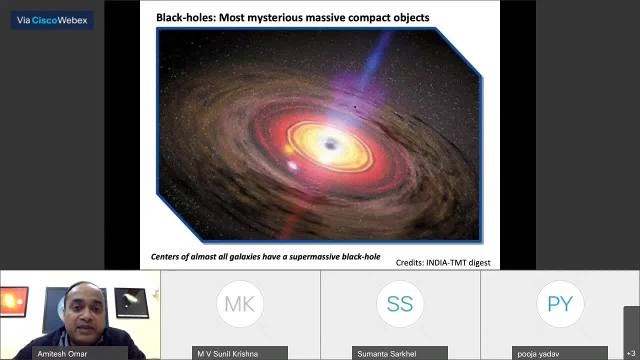 And of course we all get fascinated by some of the mysterious objects which we encounter in astronomy, particularly the black holes. And everybody you know, attention is caught whenever there is a news about a black hole. Particularly this year the Nobel Prize was about the you know establishment that black 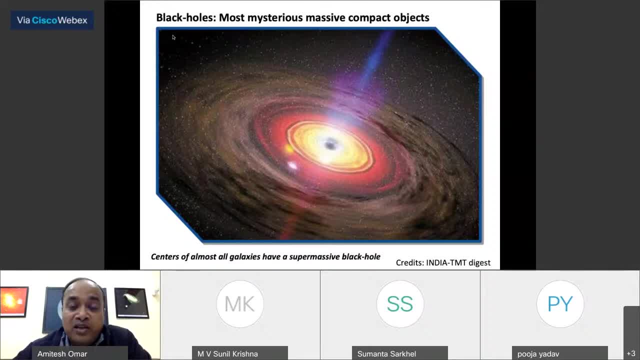 holes can exist and observationally, in the Milky Way that black hole was detected. Now we know that centers of almost all galaxies have a supermassive black hole And there are phenomena associated with that which are always in limelight in astronomy. 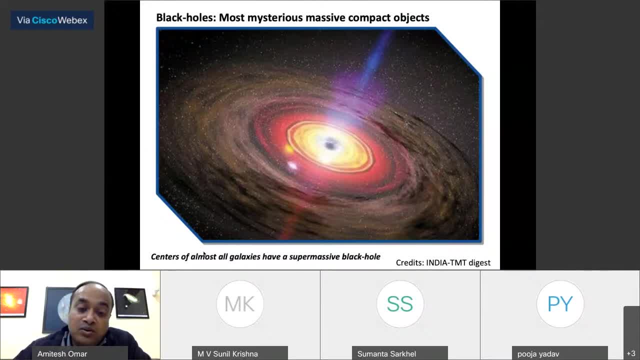 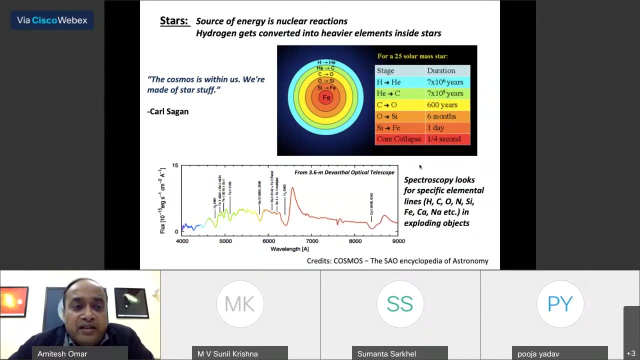 And there is a large group of astronomers who work on phenomena related to black hole, both observationally as well as on theoretical aspect. Now, of course, the stars. That's what our eyes can see, and we know that the source of energy in the stars is. 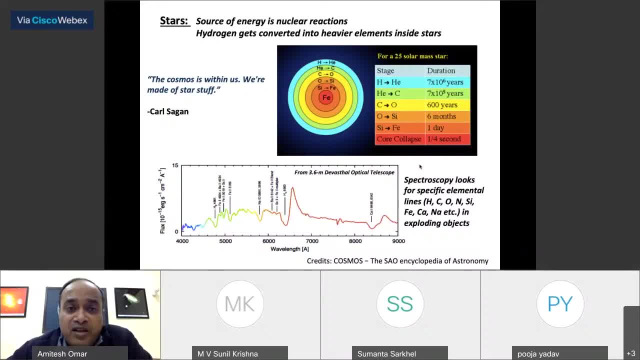 nuclear reactions and there are different reactions Here. the hydrogen gets converted into heavier elements. So the stars are basically the factory to make heavy element and we are made of heavy element. And there is a famous quote by Carl Sagan that the cosmos is within us. 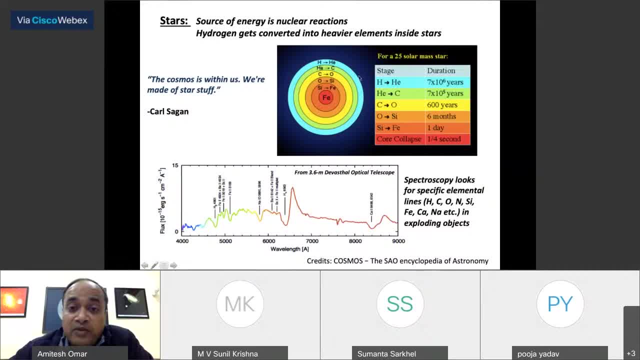 We are made of star stuff, And how that is true If you look at this picture For a 25 solar mass star, for example, which is a very massive star, 25 times the mass of the sun. they evolve much faster than the sun. 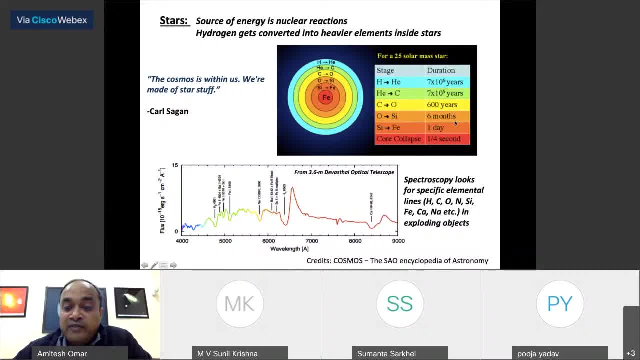 And if you look at the time scales of their, you know typical lifetime. hydrogen gets converted to helium in about 7 million years, Then helium converted into carbon in about another million years or so. Then carbon is converted to oxygen in about a few hundred years- 600 years. 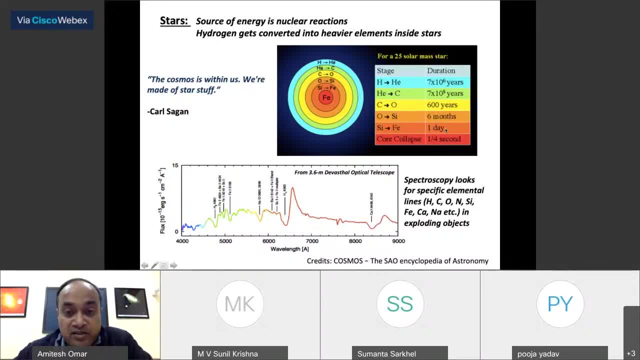 Oxygen to silicon six months, Oxygen to iron, which is the stable, the final stable core, in one day And then, finally, it cannot sustain- you know its mass- and it has to do a core collapse which is causing a supernova. 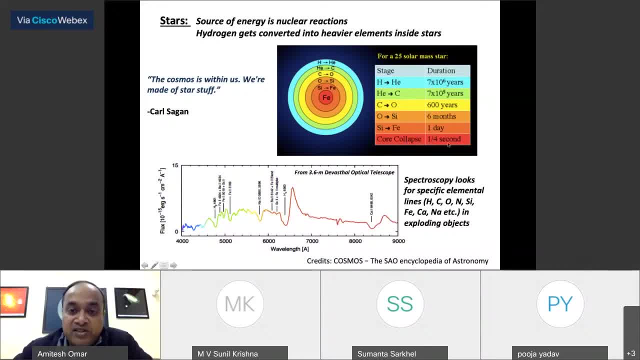 And that happens in a fraction of a second. That's the end stage of a star, And so when it ends its life, it expels out all these heavier elements which it has fought in its lifetime, And that gives rise to 4 billion years. 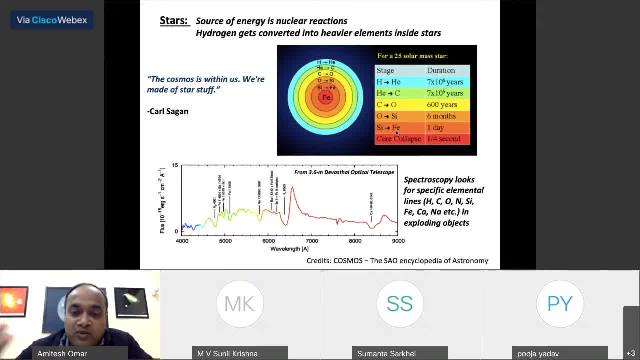 That's the end stage of a star, That's the formation of new stars, as well as the planets on which we live, and we are made of that, And that's why we call. the cosmos is within us. We are made of stars. 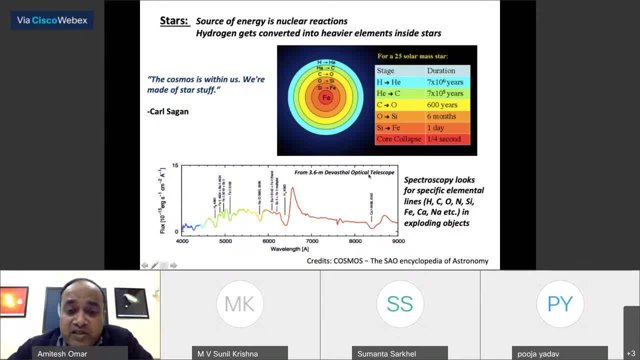 And the telescopes help that. This is a typical spectrum of such a collapsing star, taken from the Diversal Optical Telescope, And what we look here is the signatures of these elements, For example, hydrogen, carbon, oxygen, nitrogen, silicon, iron. all these spectral lines we 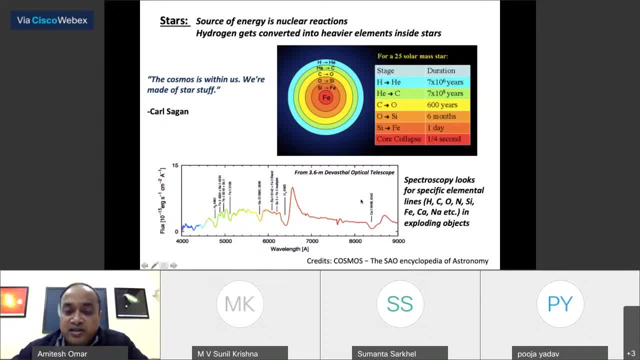 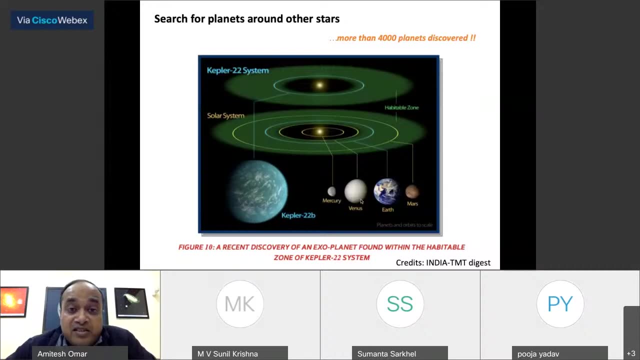 know their wavelength and they are detected. And that's what astronomers in fact do when they look at such objects. They try to estimate how much you know these heavy elements or dust has been formed. There is another very exciting area. that's searching for the planets around other stars. 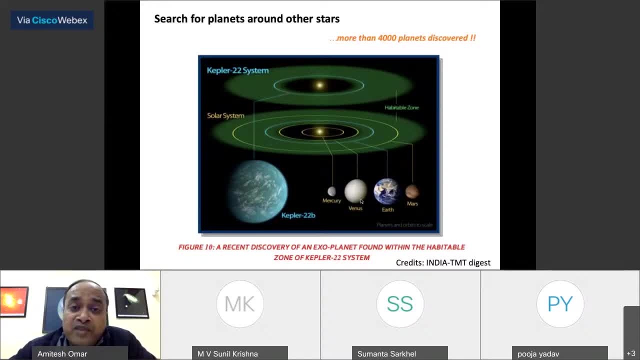 And that tries to answer the question: are we alone in the universe? Of course, we still do not know the answer- Are we alone in the universe? But there is a very high chance that there are planets. Similarly, there are planets. 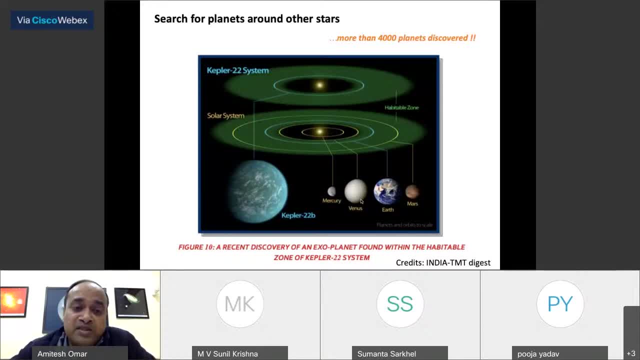 Similar to Earth around other stars And this is one of the pictures which came several years ago in limelight, that around another star a planet was discovered which has in a very similar habitable zone what we see on Earth. 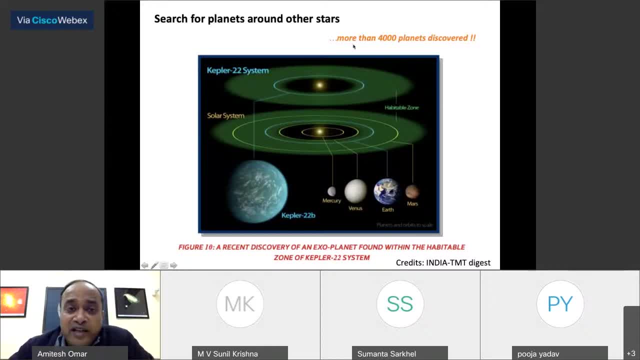 And now we know that there are more than 4,000 planets which have been discovered. In fact, it's said that it's difficult to find a star which does not have planets. Every star has a planet. Every planet has a planet. 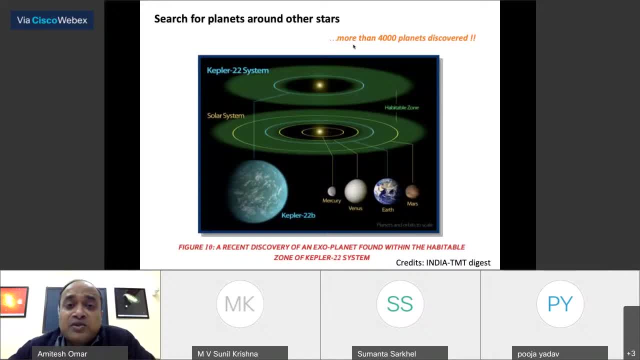 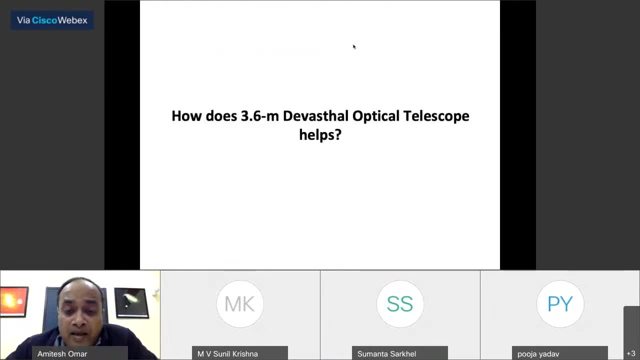 Every planet has a planet. When we are supposed to have planets, it just, you know, we have to discover them, And that's a very exciting area where astronomy works. Now, I'm sure you have in the previous- you know, in the same series previous- talk heard 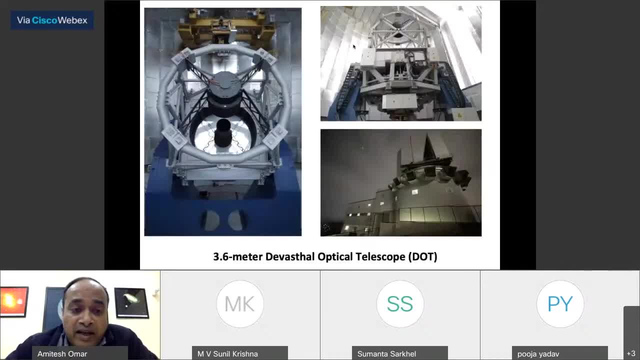 about the Devastar optical telescope. And that's the picture of the optical telescope. What you see here is the primary mirror of the telescope. This is the whole structure And this is from the outside. It's been used for finding these planets. 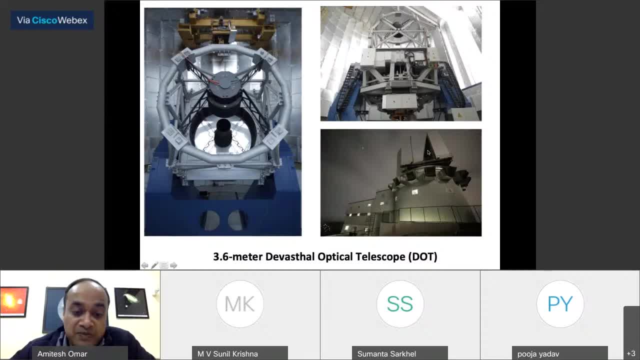 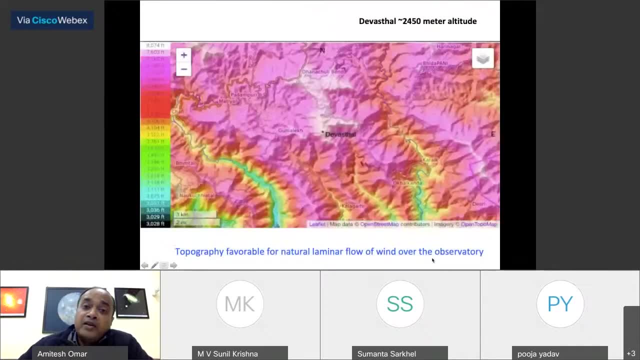 which the telescope is housed. we call it as a diverse optical telescope, or dot. very interesting thing to look at that a divestel is very close to, of course, the place i am sitting. it's just about 20 kilometer line of sight, uh, from nanital, and if you look at this topographic map, 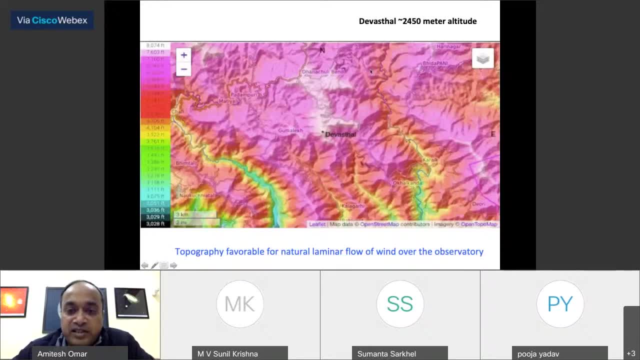 where the altitude is color coded in the whole region around divestel. divestel is the highest peak in that region and, very interesting to note, there is a sharp form. in fact, this is the plain area, the the south and this is the north, and that's what makes us, you know, makes the site a very 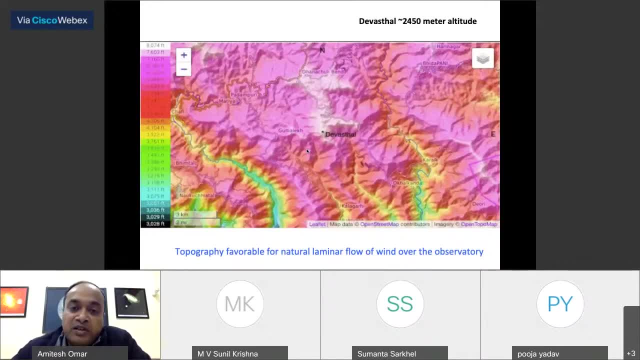 well suitable for making optical astronomy, because optical astronomy is affected by the turbulence in the atmosphere and we want to minimize the turbulence. so the site selection is going to be very important in any any you know- optical telescope placement, and it turns out that this local topography is very much favorable. 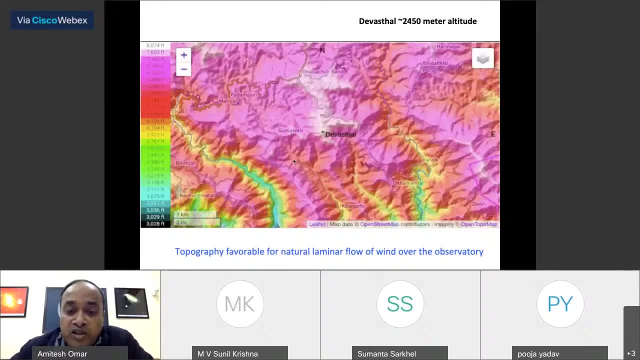 for maintaining a natural laminar flow of wind over the observatory. so the wind becomes turbulent after it passes the divestal peak, and so if you place the telescope here- that's what we have done- there is very little interference from the turbulence which air generally creates. 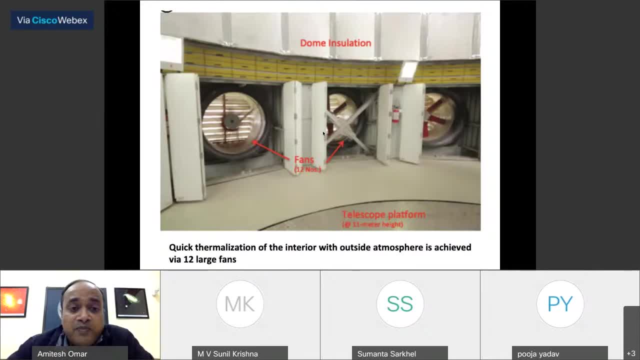 so we also make additional arrangement in the telescope that it's well thermalized from outside into the interior, because there is, if there is any thermal gradient in the building that is going to give right, that is going to, you know, affect the observations, because then there will be a heat. 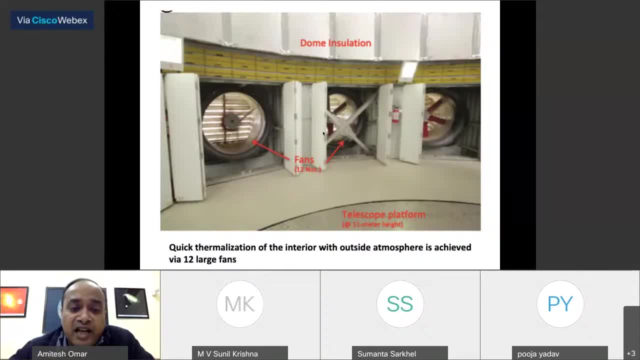 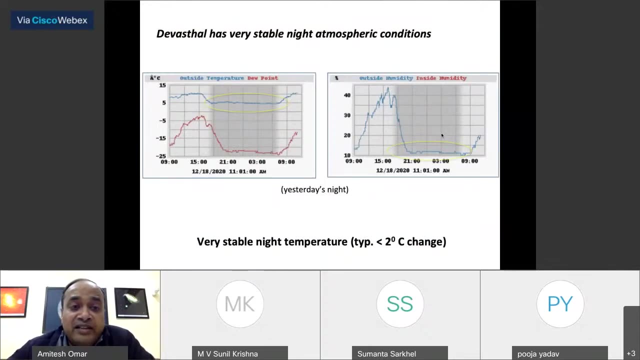 transfer and the turbulence will be created. and so there are these large fans which help in the observatory. they are switched on during the observation as well as before the observation, to interior, with the outside atmosphere. in fact, this i really just saw, it's from yesterday's night. 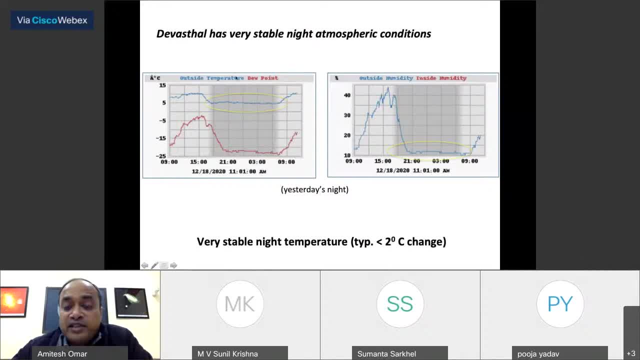 that what has been the meteorological parameter there? you look at the outside temperature and humidity. look at the stability of the temperature: it just whole night it is stable at five degrees. okay, very little variation in the temperature. and look at the relative humidity: is close to ten percent and very stable. it does not change. so it's a dry place, at least in these months. 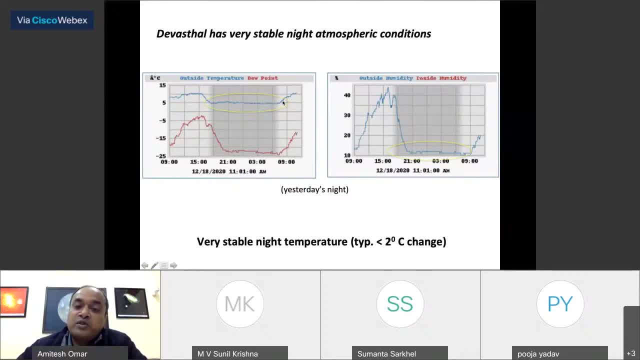 and very stable light temperature, and that's what we call the astronomers dream for any site. this is a perfect example of a you know, a textbook example of a very good you know astronomy site: very stable night temperatures and that gives rise to very little turbulence over the night and that helps. that helps a lot, in fact. if you look at the 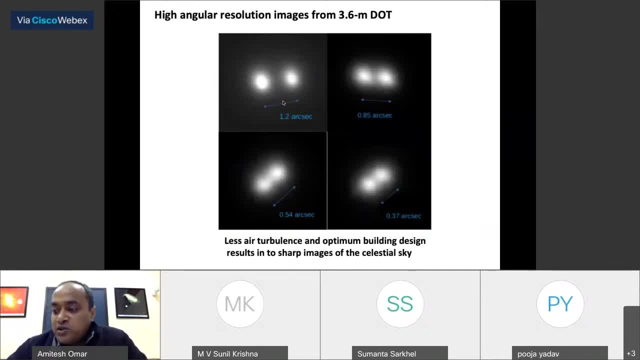 images which we get from point six meter. they were still optical telescope. we see a star separated, very small angular separation. in fact most are the good observing sites typically achieve one to one point five arc. second, you know that that these two sources which can be resolved in this sky, they will still can actually resolve sources. 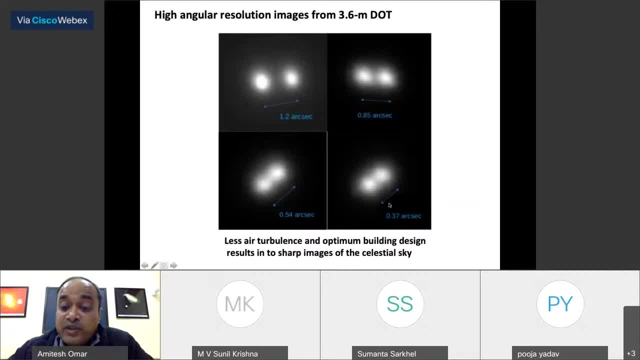 these are two stars, binary stars, which are separated only by about point four, arc second, and that's really very good side. some of the best observing sites in the world actually achieve this kind of ground-based, you know, observatory about point four, arc second. in that places they were still at par with many big 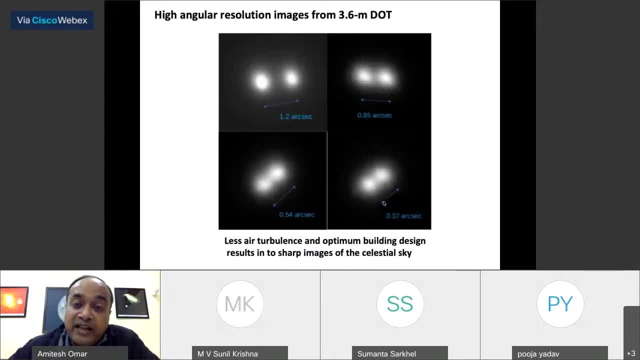 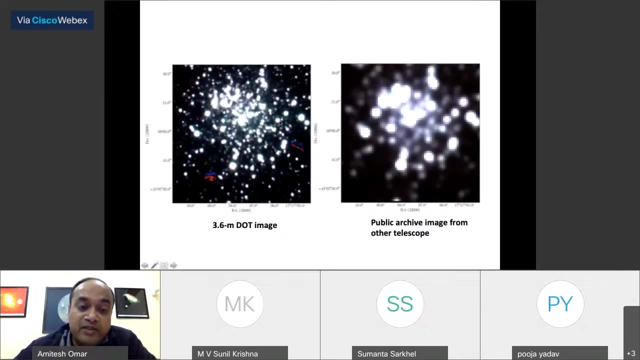 international observatory sites and that is because, again, as I said, that it's air turbulence is less in the building, which has been designed very optimally, and that results in the sharp images of the celestial sky. in fact, you can see the example here. this is the image on the left taken from the Devastal optical telescope, and right 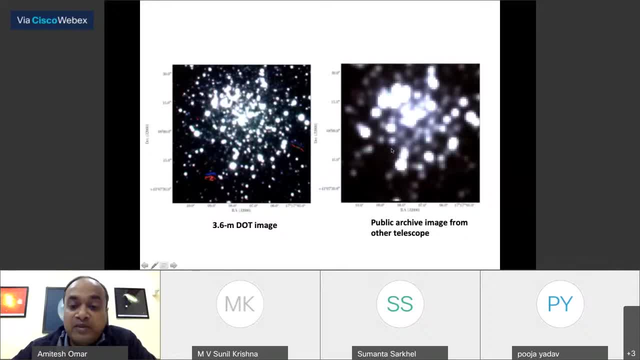 image is the same image but previously available from the public archive, which is really available. anybody can download and do signs. so now you see that there is a huge difference between what is previously available publicly and what we are achieving here. you see number of stars, the resolution, in fact everything. 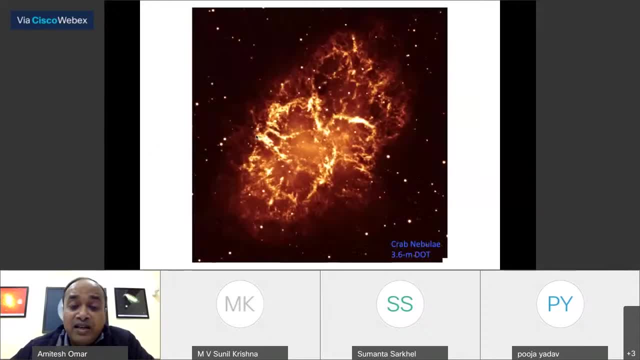 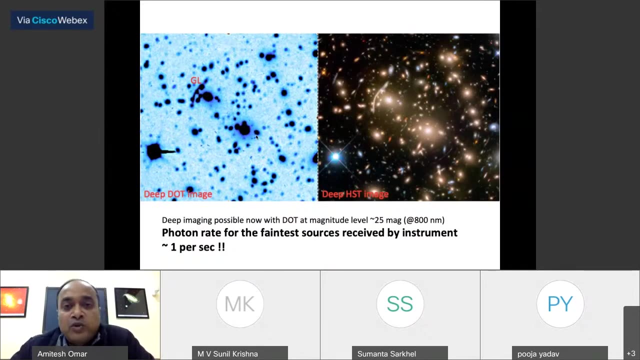 is sure so sharp here and that's just another eye catching image of the crab nebula, very sharp image. that's what we get from three point six meter. now it's just not the sharpness. the site is at a remote place and it is quite dark. there is not much, you know. there are not many houses, they're not. 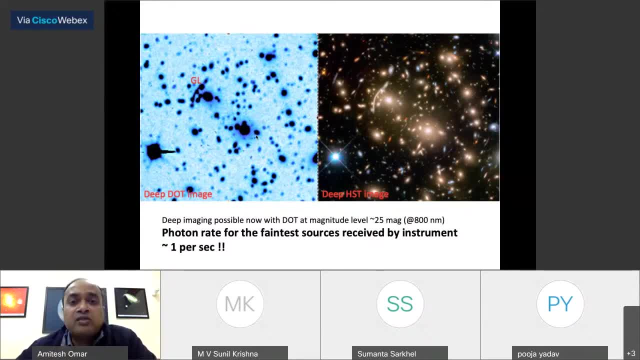 you know, as you know, the otra can hills are not very much populated also and so it makes the dust decides very dark. in that helps to achieve very specific, small, you know, photon rates detection. so some of the sources which we have detected. so this is for a comparison with the hst image. the comparison is made to see whether the faintest 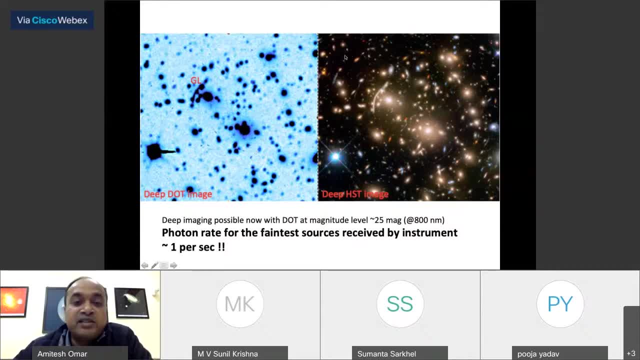 object detected in our image were detected in hst image or not. in fact we did. of course, hst image is much deeper than what we get. that's because hst is in the, you know, outside the atmosphere, in the- you know- the most favorable conditions. some of the objects which we detected 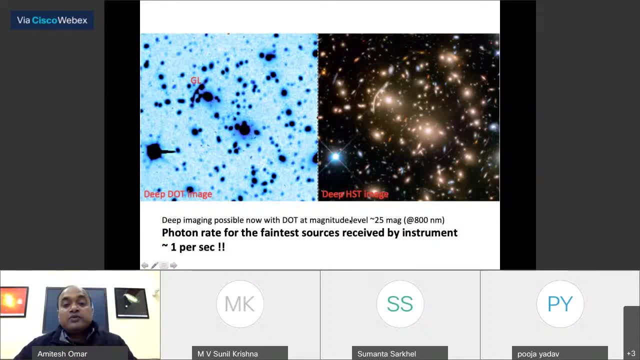 in this image, for instance, they reach to a magnitude level of 25 magnitude in around 800 nanometer movement. and that what is the magnitude scale here? if you just convert it to photon rate, that is about one photon per second. that's a very, very feeble. you know, very low photon rate. what we can detect from the sky using this telescope. 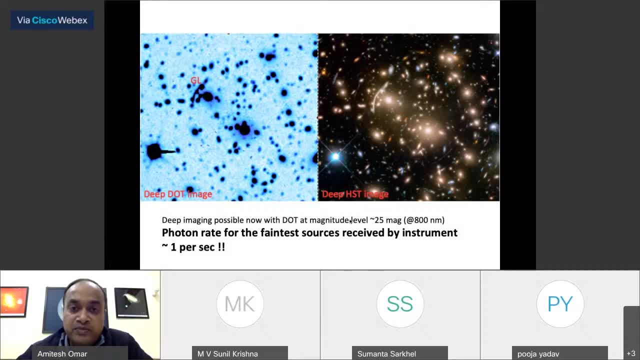 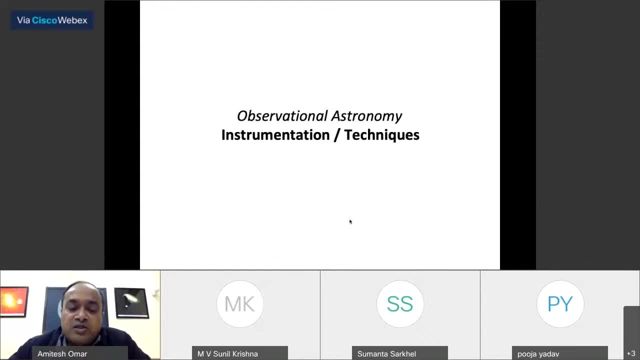 and that was previously not possible with any indian telescope to achieve. now let me come to the. what are, you know, the observational astronomy, what are the instrumentation things, what are the techniques that people use, or you know we use, and where are the opportunities to join that? the telescopes, the modern telescopes, like 3.6 meter top. they are pieces of engineering marvel. 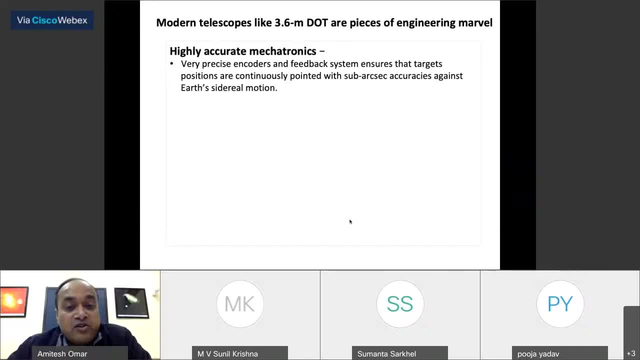 why so? first thing is that it's a highly accurate mechatronics. it's a mechanical system as well as electronics, and they talk to each other, they provide the feedback and they have a very precise encoders. they have a very precise feedback system, very sophisticated, and that ensures that the target positions in the sky. 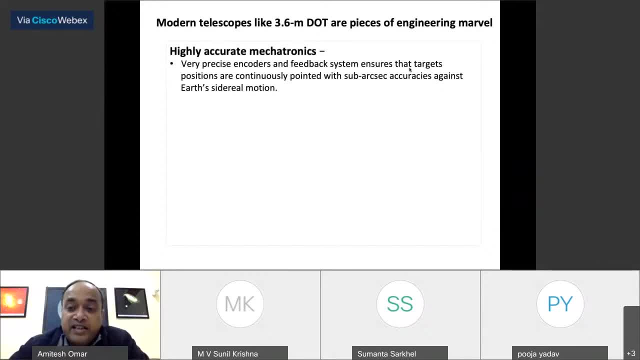 are continuously tracked, pointed and tracked with sub-arctic inaccuracies, because the earth's sidereal motion is changing the positions of the stars continuously and we need to track them with sub-arctic inaccuracy, and that's basically possible because of a very accurate mechatronic system. 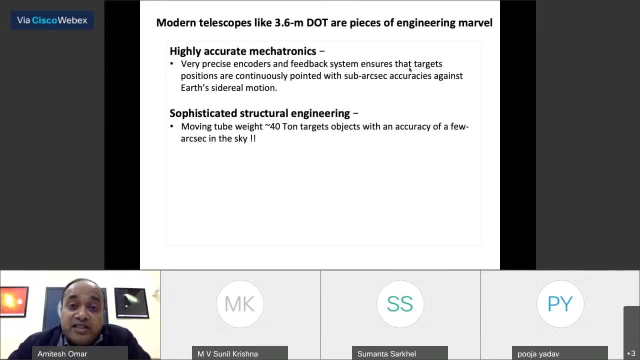 then there is a sophisticated structural engineering. remember that this telescope, like 3.6 meter, is a very heavy telescope- it's more than 120 ton- and the tube itself on which the mirror and the instruments are mounted they weigh about 40 ton. okay, and that 40 ton tube moves with a very- you know, very- precise accuracy and it also targets the 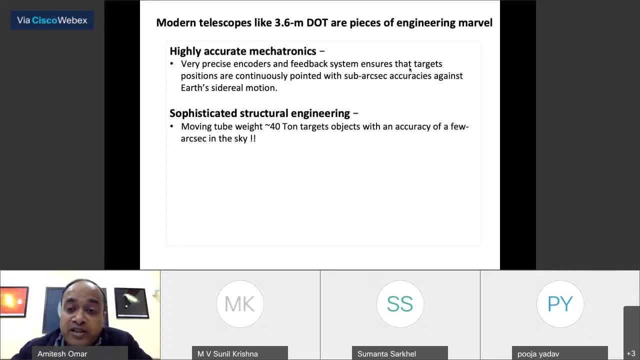 objects in the sky. so you ask the telescope to go to an object, typically it will bang on. it will go there with highly, you know uh, accurate, not more than a few arc second. you know errors, and then it starts tracking with sub-arctic inaccuracy so you do not see, you know, any effect of the earth. 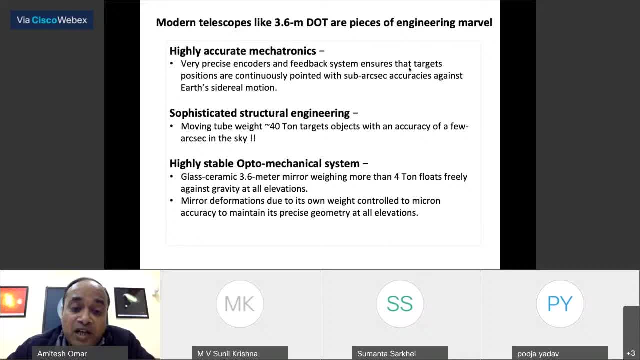 rotation in that. and then a very stable optomechanical system because, remember, this is also a large mirror, 3.6 meter mirror itself weighs about four tons, four, 0.3 ton to be exact, and it needs to float freely against gravity at all the elevation the telescope. 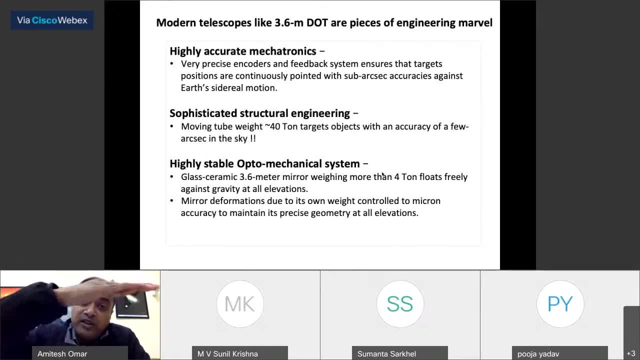 can look at very low elevation, like 15 degree, you know, from the horizon, and of course it can go anywhere in the direction, any direction, and that weighs. the mirror itself weighs about four ton and that needs to be controlled if it should not receive any residual forces of the gravity. 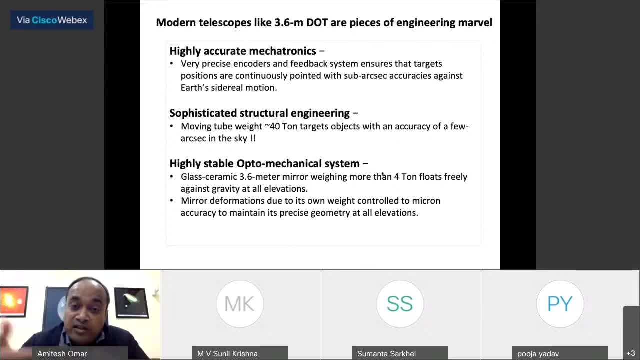 otherwise the shape itself will distort by its own weight photon structure, and so there's a very precise optomechanical system built in, and the mirror deformations are controlled continuously to micron accuracies so that whatever is the shape required to get the best focus. let's say: 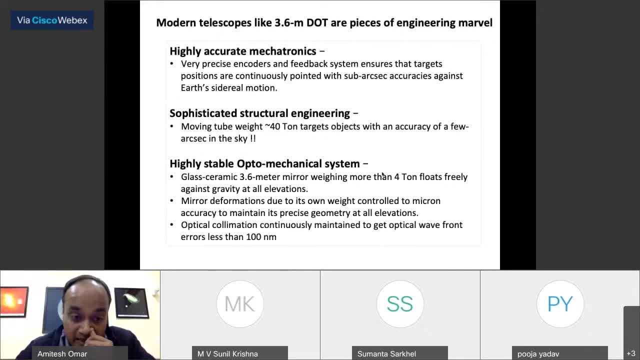 the best optical collimation is achieved by this system. and if you look at the numbers here, the optical collimation between various, you know the optical systems, you know the optical systems. and the optical collimation between various, you know the optical systems. there they are continuously maintained to get optical view front errors less than 100 nanometers. 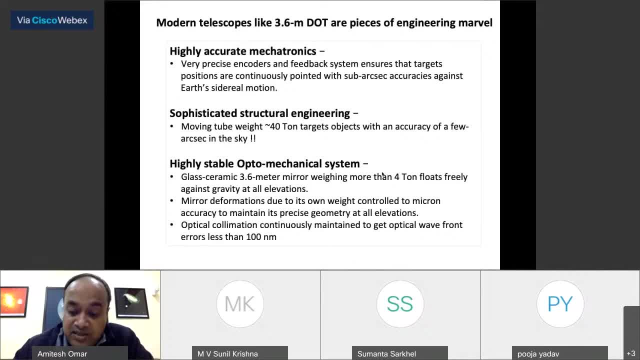 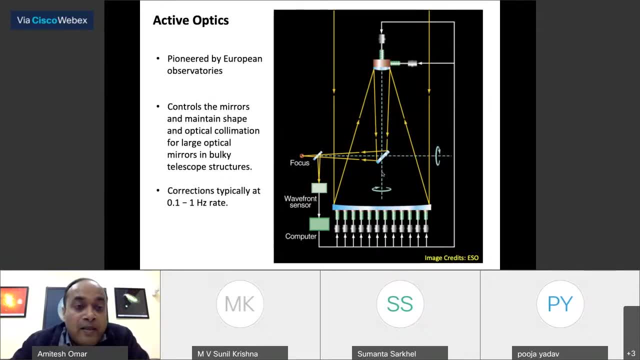 and that's because of a very precise system built in and what we call as active optics. without active optics this would not have worked. what is active optics here? this is actually pioneered by European observatories. it controls the mirror and maintains shape in optical collimation. for large optical mirrors in bulky telescope is that you remember as the telescope? 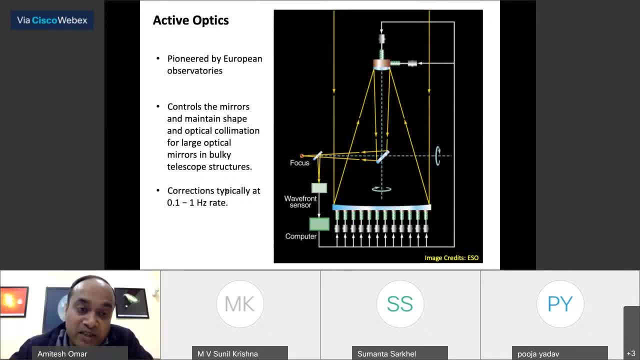 become larger, the structures also become large, very bulky, and so there are mechanical flexures, there are mechanical inaccuracies, because we cannot achieve, to you know, like a micron accuracy in such large mechanical structure. so this is achieved by a technique called active optics, where the view front is sense, the light which is coming on the telescope, part of that is received and it's 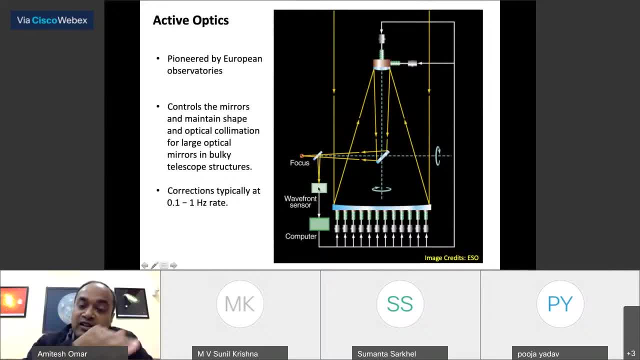 a view front. it sense that. okay, whether it's a flat view front or there are curvature or variations in that. and it's a view front. it sense that. okay, whether it's a flat view front or there are curvature or variations in that. they are assessed and they are fed into the computer and then mirror sits on what we call. 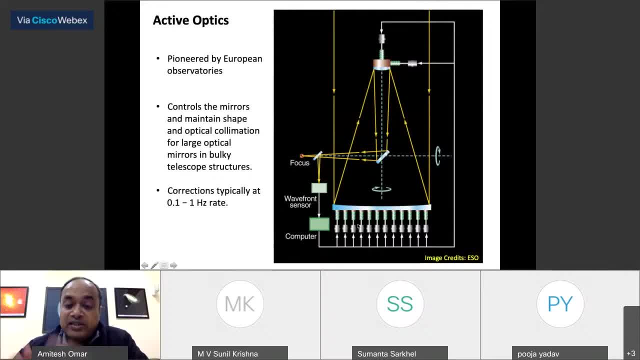 the actuators, pneumatic actuators they are. they basically push or whatever is push is required so that mirror is always floating. the same system also gives a feedback to the secondary mirror system, because normally to fold the optics- what we call the folding optics- to to keep the size. 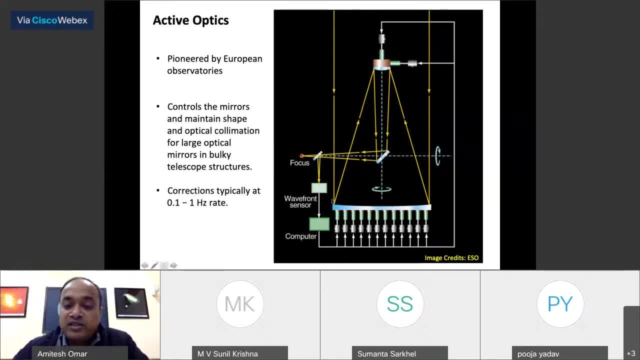 smaller. we usually maintain two mirrors. so this half of the you know part of the collimation is the other part. the collimation is done here so that the telescopes become compact. so these are two mirror system and they both are controlled for, for example, the flexure against the gravity. 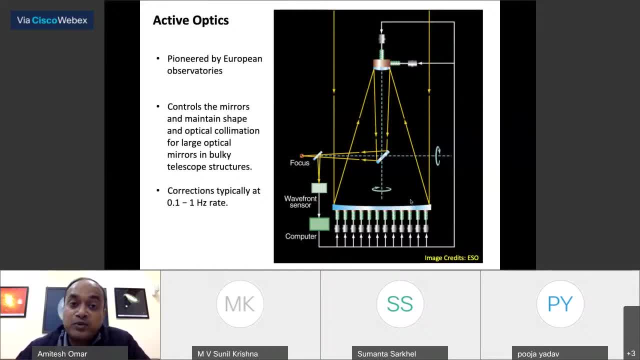 sometimes again, the wind also and also the change in the temperature suppose temperature changes, and so the material expand and contract, and that itself will make the images really go out of focus, and so that is continuously maintained by the system called the active optics. these corrections are not very fast corrections, they are typically. 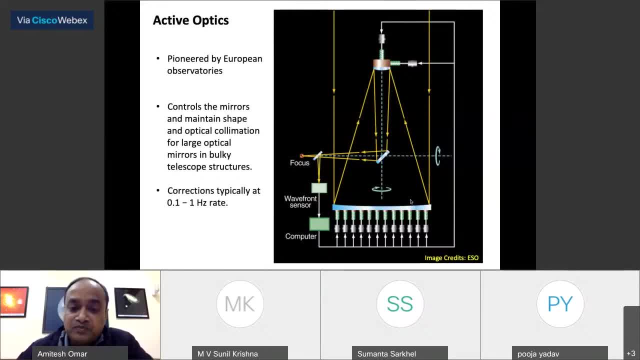 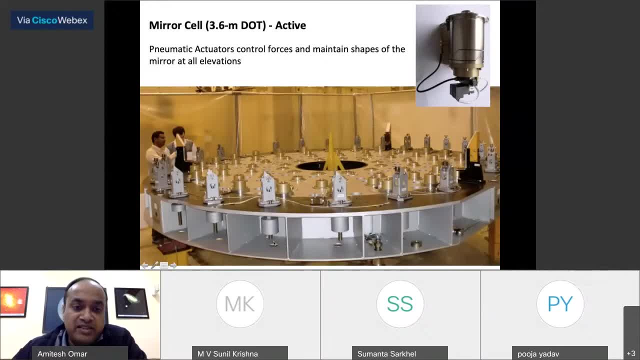 required at about 0.1 to 1 hertz rate, and this is the picture which i really like people to see- is the mirror cell. these, these are the cells under which the mirror, the 3.6 meter mirror, sets, and these are controlled by pneumatic actuators. what you see here are the actuators, these golden 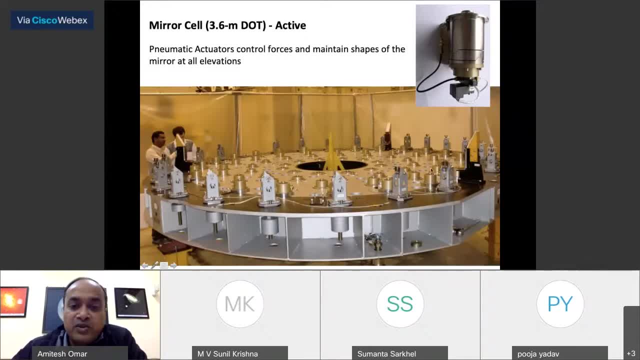 pieces, and then there are also this support system, so these are adjusted and then they control the mirror to very high accuracy. they are in fact, they are very high accuracy. they are very high accuracy. these pouvez are sub newton. you know it's about point one, newton: accuracy. they can. 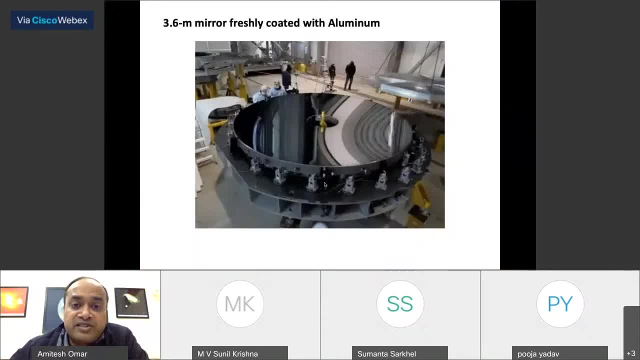 maintain the mirror shape and when the mirror is put. this is the picture at the vesnel. mirror is coated. because the mirror is in the open, it receives the dust all the year when we make observation, so the mirror is carefully brought down from the telescope. it's clean and 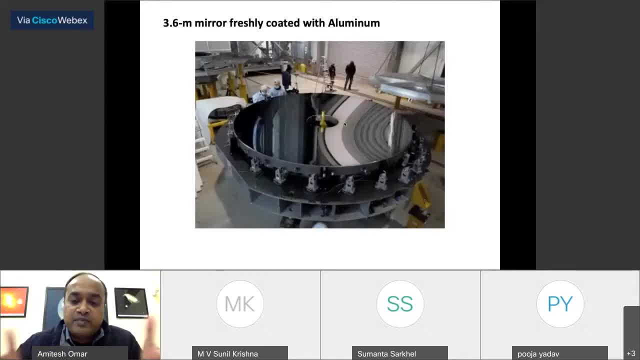 it's recoated with aluminum in the facility and then it is remounted in the mirror cell. once mirror is mounted in the cell and the cell is made active, it is ported to the against the mirror cell. the mirror actually floats, It is. there is no residual forces from the gravity, so that it 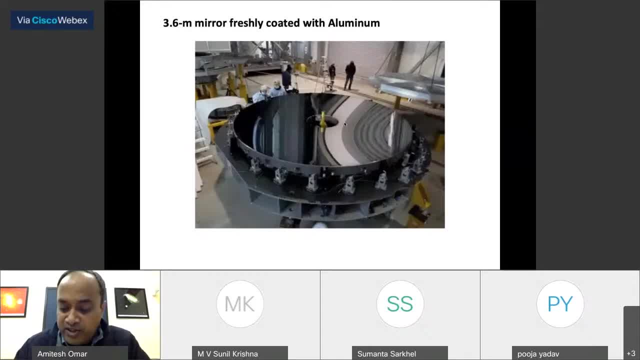 doesn't deform. That's something maintained at a very high accuracy. If that is not so, the mirror itself, as I said, will deform and we will not get very sharp images, which we saw earlier. Similarly, there is a secondary mirror support system because we need to adjust it. 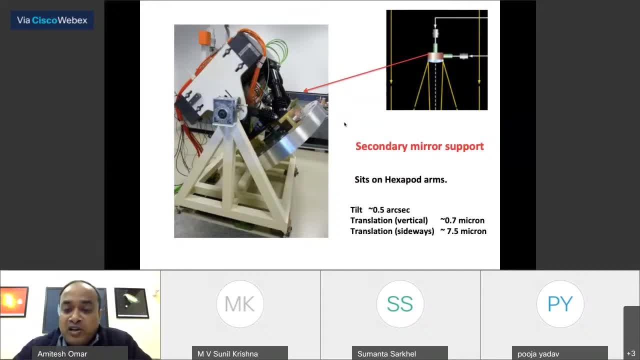 continuously and that sits on what we call the hexapod arms. And that hexapod arm is also very precisely controlled. For example, its resolutions are that it can. it can do six motions basically. So there is a lot of. there's a translation in the vertical sideways. There are 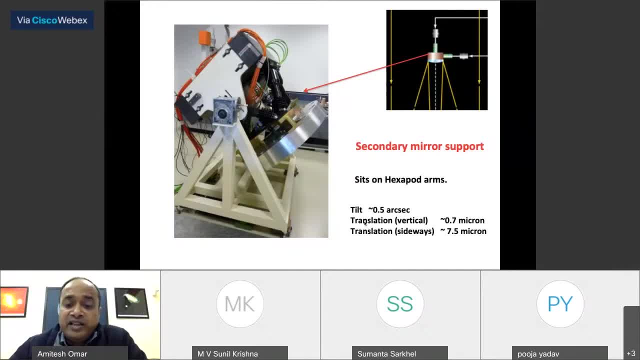 different directions tilt, and that can be done with an accuracy of about half a second. Translation can be done at about sub micron and there is another translation about few micron. So this is depending on what is the requirement from the system, And these are really sub micron and sub 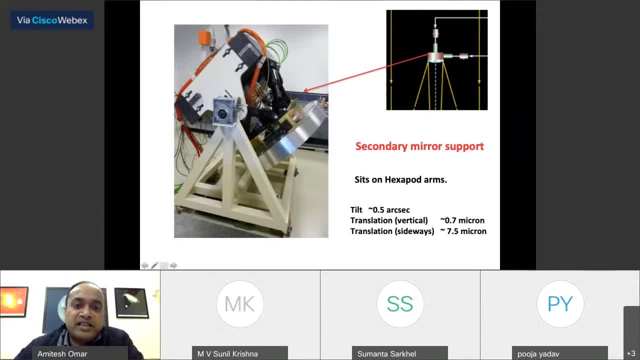 arc second accuracies. So what is really to appreciate is that these are bulky system and we need to really control them at a very sub micron accuracies. And that's what these modern systems, you know, achieve. that Without this large making, a large telescope is completely impossible. We just cannot. 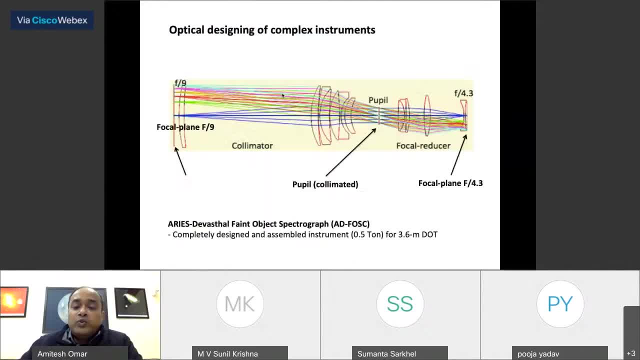 collimate the large optical telescopes. We also take part in optical designing of complex instruments, instruments, particularly the instruments which are going to be used in the future. One of the instruments which we have designed and commissioned now, and in fact presently, is being used by 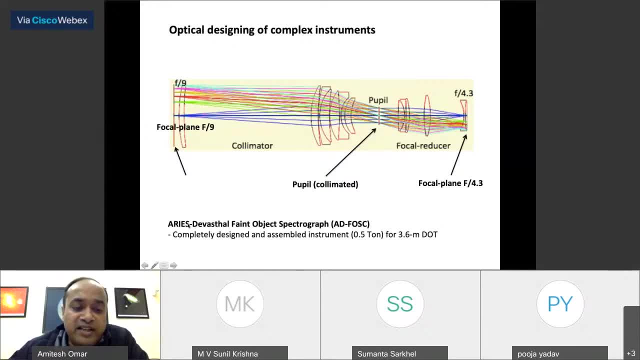 astronomers is the EDFOSC. It's called Aries Devastal Front Object Spectrograph and Camera. It's completely designed and assembled by us. It's about half an instrument. the optics is large and this is a normal collimation and then pupil and then focal reduction. So this is very precise, you know. 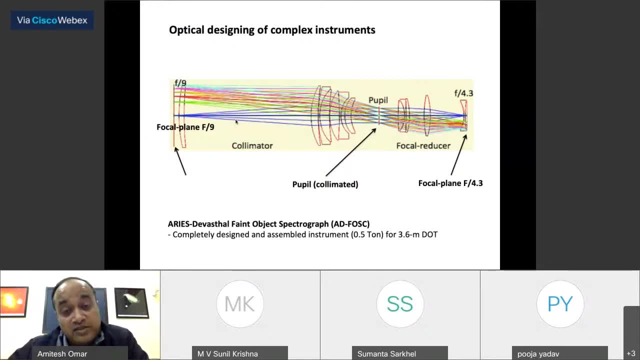 uh thing, because we do not want the optics to distort the images, because telescope is producing sub arc second images and so this also should match with the sub arc second resolution, and so it becomes really complex optics. we have to put multi-elements optics so that the image quality 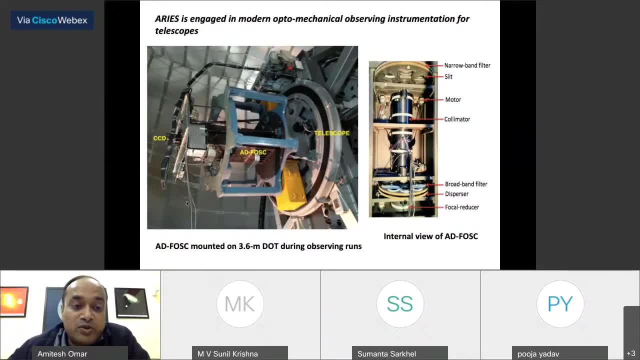 is maintained. now this is how the instrument looks like this. this, at first, is mounted on the telescope 3.6 meter backing and it's you know it's really working there. but if you want to look at the internal structure, there is a lot of optics. we can exchange the optics with the filter, with the. 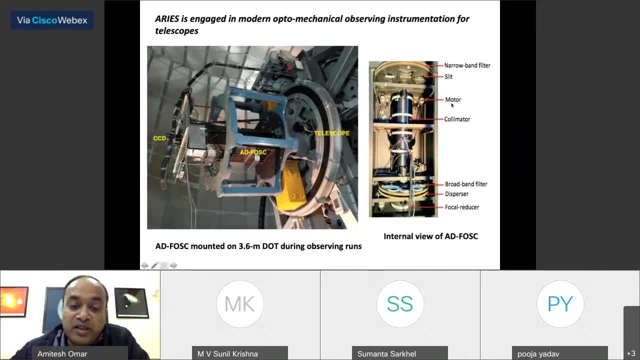 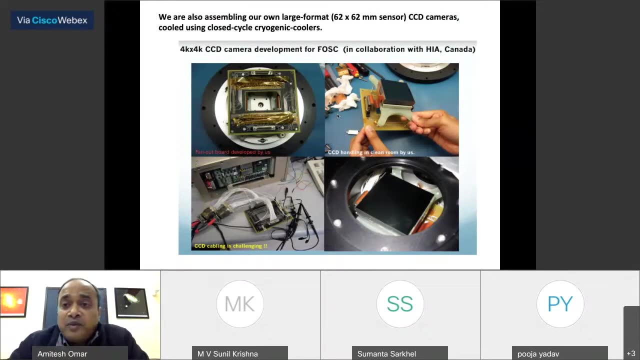 fridge gratings, because we can also do spectroscopy in this instrument, and so this is all precisely controlled uh by, you know, the computers, and this is mounted. we are also, uh, taking part, and we are assembling our own large format ccd cameras. now, ccd camera is in fact not something which is very. 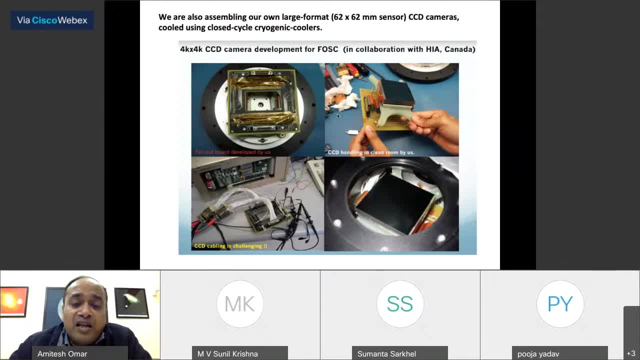 common in our country. most of the ccd camera we import- and there are always issues- that they are very sophisticated instruments and if there is any issue we have to send it back and that's really a very long time, apart from the money which is spent, but it's a- the time loss is really large. so we 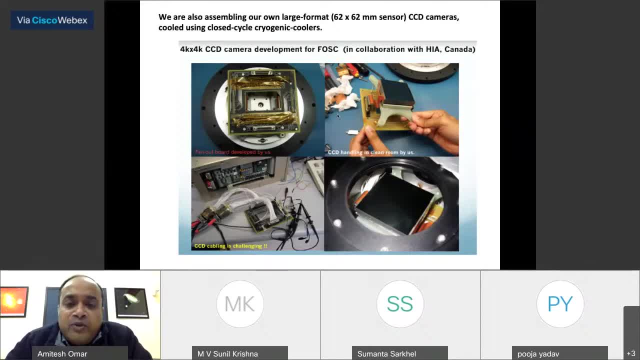 started this program in collaboration with the hia, canada a few years ago and now we assemble our own ccd cameras. we maintain it here. if there is any issue, we solve it within, you know, a few days or a few hours, depending on how complex the column is. so we can handle these very- uh, you know sensitive. 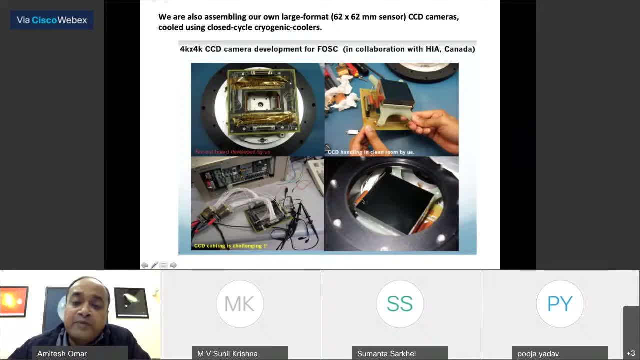 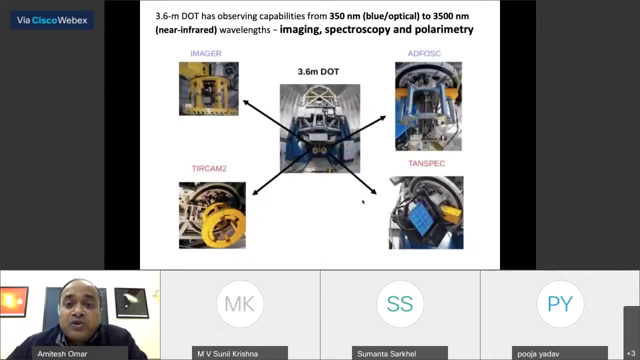 devices in our lab. we are in an anital. in fact, the camera which we are using in 3.6 meter, the western telescope in the atfos, is made here and these images which i showed you, some of the images are taken by this camera which we built here. now, dot has got many instruments. of course it has a 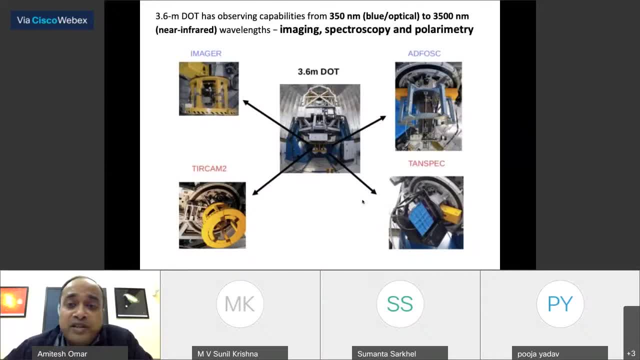 capability to observe right from the blue 350 nanometer which is passed from the atmosphere below it- we cannot do from ground-based observatories. and then up to 3500 nanometer, that's the near infrared, or 3.5 micron give and we can perform imaging. so there are instruments like 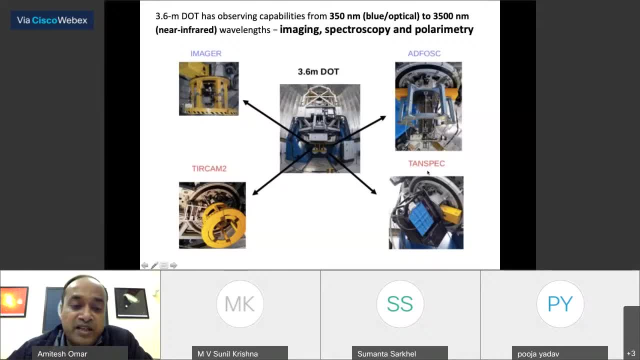 imager and atfos can also do imaging. then there is a 10 spec and tircam. these are near infrared instruments, particularly, i mean, designed for a wavelength above one micron, and so they all can do imaging spectroscopy now, as well as the polarimetry, the polarization is also important. 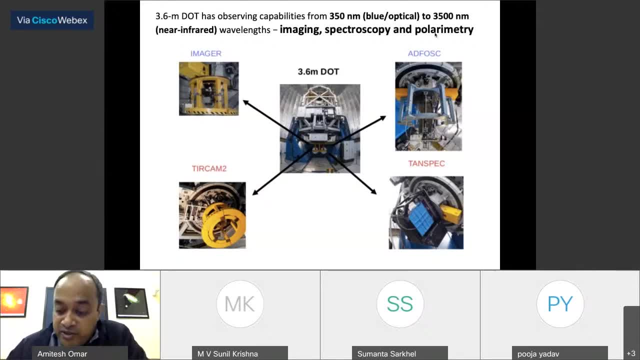 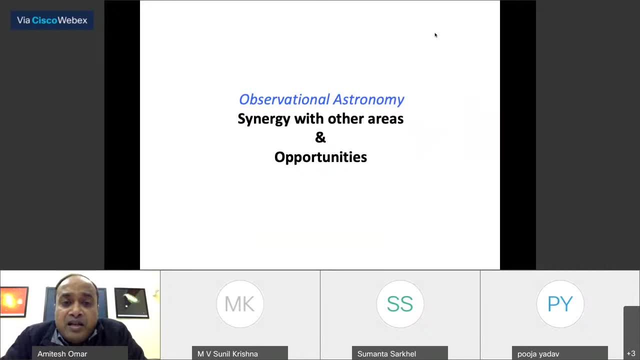 to measure the astronomy and we are including certain polarization, you know, instruments in that. now, coming to the last part of my talk, that what are the areas where we can sort of have you know some collaborations- multidisciplinary or interdisciplinary areas- and what are the opportunities for students? 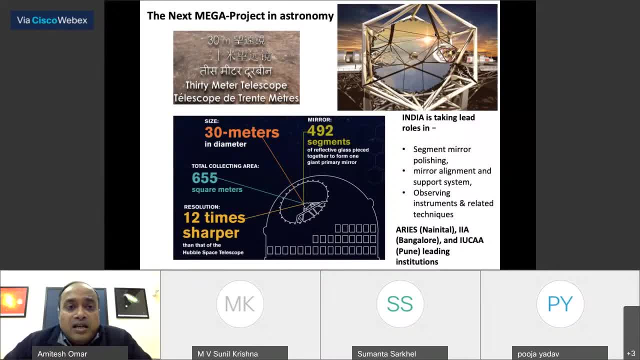 let's see, and let me bring you to this: the next big thing in astronomy is in optical astronomy is one of these mega projects is called 30 meter telescope, which will be the, you know, world's largest telescope in future, in coming years, and its size, as you see, is 30 meter, going to be 30. 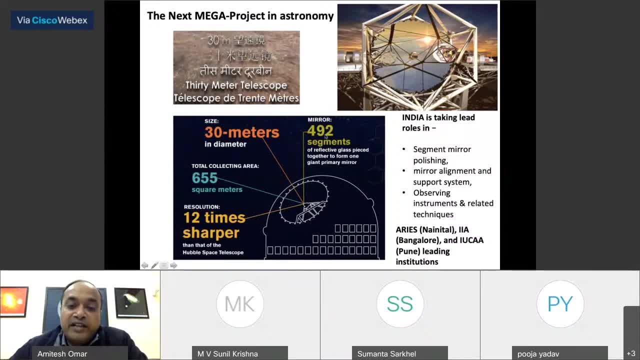 meter segmented mirror pulsing. there will be 492 segments of reflective glass which will be, you know, sort of stitched together and they will be maintained a required geometry. so the it will make a size of 30 meter and it will be having a total collecting area of about 600 square meters. 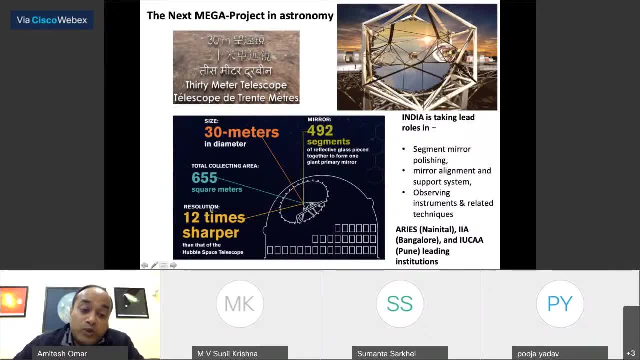 and what is the target here is that this will achieve 12 times sharper image than what we are achieving with the hubble space telescope. we know that hst is producing the best images in terms of resolution, and some of the ground-based telescope with adaptive optics. 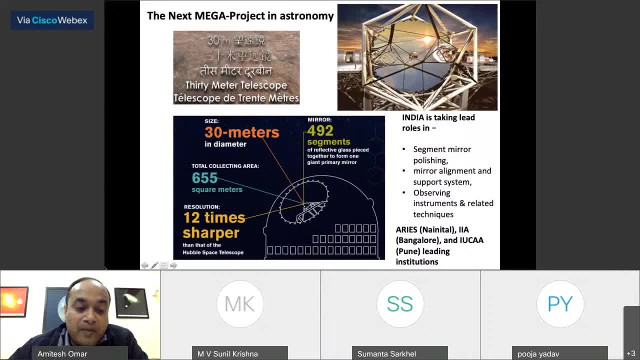 which i'm going to come in a moment, another technique. so this is going to be really changing. you know how we do. optical astronomy in india is participating in that among from other countries, several other countries and india is participating in segmented uh mirrors, polishing that this meat are pulsing facilities in bangalore maintained by indian institute. 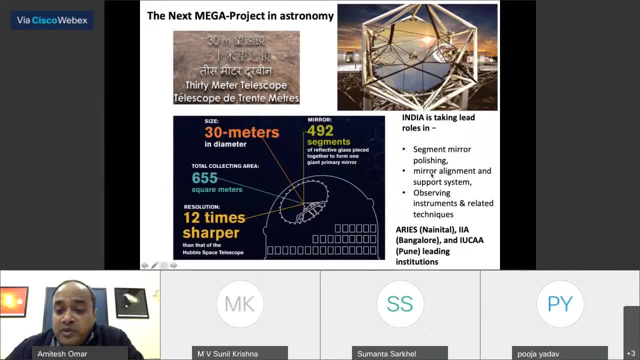 of astrophysics, there is a work going on on mirror alignment and support system, because these alignments, all these facets, have to be aligned so that they maintain the right geometry all the time. ёр alignment: all these facets have to be aligned so that they maintain the right geometry all the time. so that's also a dynamic balance of how it will be, how to maintain the vosglal encounter. so it 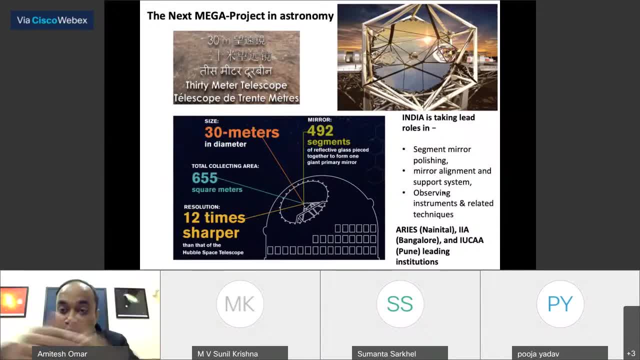 system like what we saw in the active optics. it's slightly more advanced than at the optics. then there are observing instruments in related techniques, because we have really nobody knows, you know, exactly how such a large telescope will behave and what kind of instruments issues will come. so it's not just the 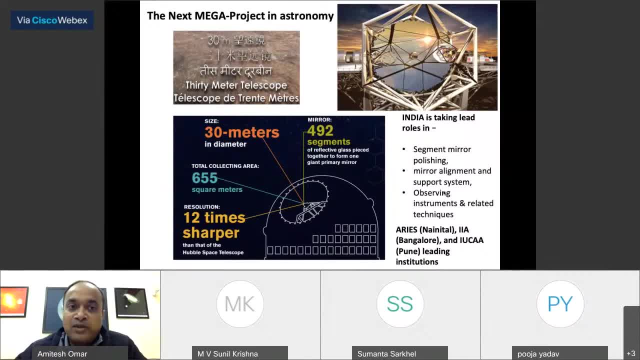 copying of old instrument. there has to be a new technique which has to be developed, and that's why it's a multi institutional, multi country collaboration. you know program and we call it to one update. you know mega project, ambitious project for astronomy in areas also participating in that. 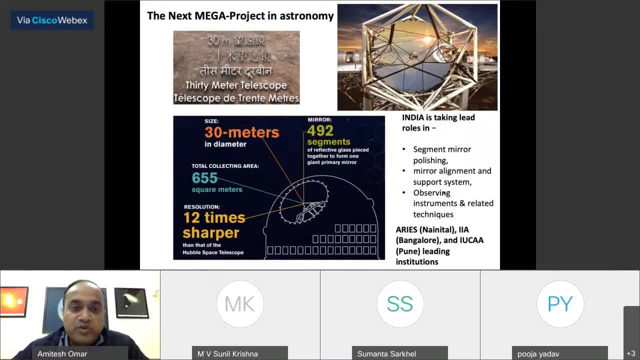 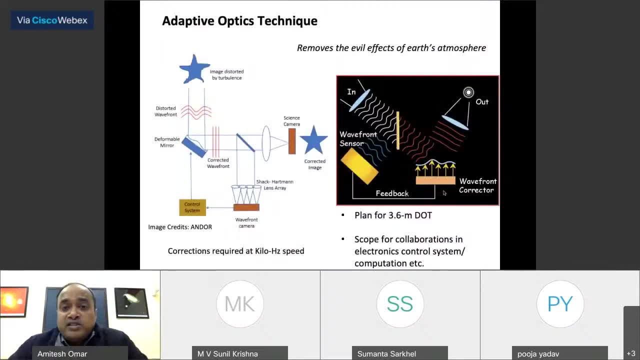 along with the IIA in Iuka, where a lot of instrumentation work as well as the science planning goes on. now, one of the thing which actually does a wonderful job is the adaptive optics tactic. now, of course, we know that the, the atmosphere, the earth atmosphere, distorts the images. 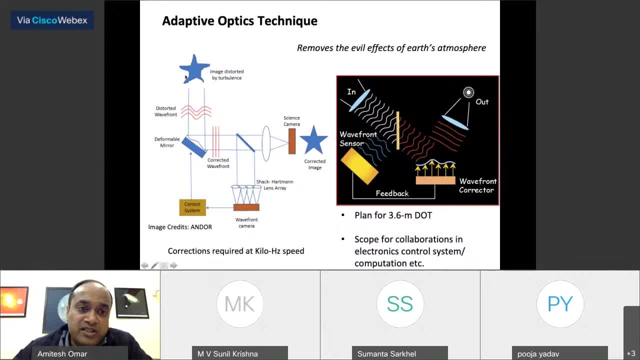 so this is a cartoon which is shown here- that suppose there is a image which is distorted by turbulence in the earth atmosphere. if we can sense it's a wavefront. so this- let's look at the right hand side thing which is a better representation of the entire thing that when the wavefront is coming part of. 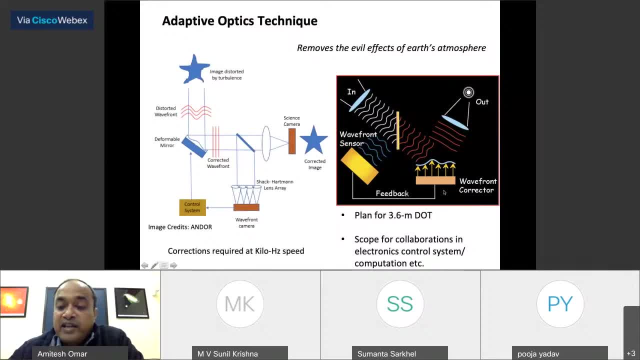 that you take it out, sense it and feedback it to a wavefront character which is actually a deformable mirror. it's a fast deformable mirror and it basically maintains the shape which is opposite of the wavefront, so that the outgoing different becomes flat. what it should have been if 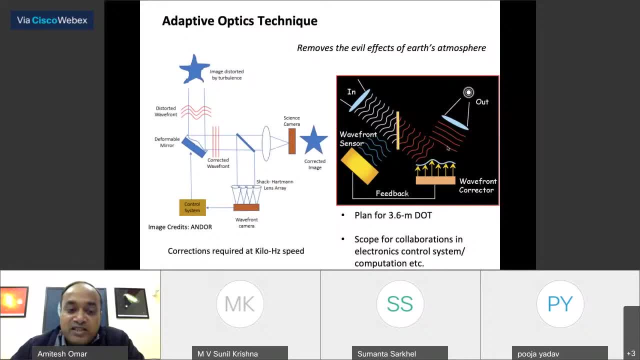 we observe it above the atmosphere, and so this correction needs a very fast, you know, kilohertz correction, because our atmosphere has scales, changes on the scales of milliseconds or tens of milliseconds, sometimes few milliseconds. so different layers of the atmosphere have different time scales and we have 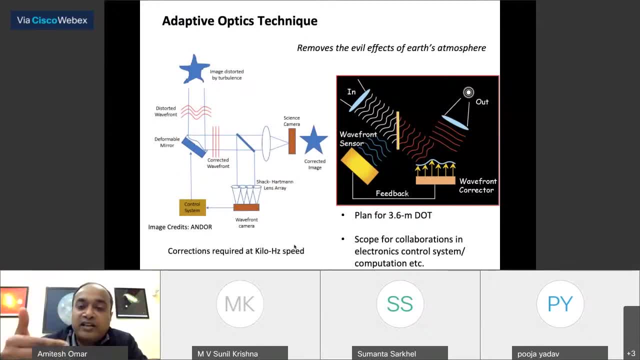 to basically sense the atmosphere, and we have to basically sense the atmosphere layers and keep on correcting in the real time so that we get an image finally, as if we have obtained the image above the earth atmosphere. and that requires a lot of. you know techniques as well as modern. you know technological. 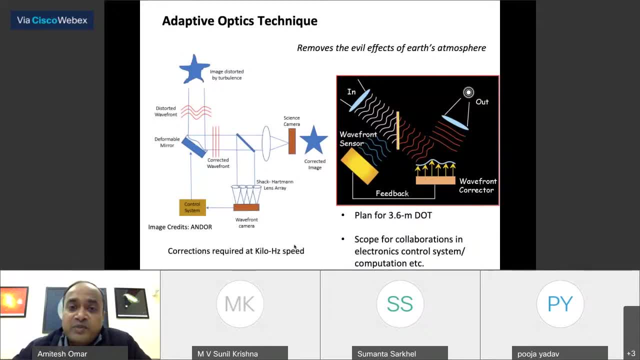 challenges and we are putting up a plan for 3.6 meter dot in here. I was definitely like that. there is a large scope for collaborations with engineering and technology Institute's and students and faculties. who are, you know, interested in designing fast control system? if so, 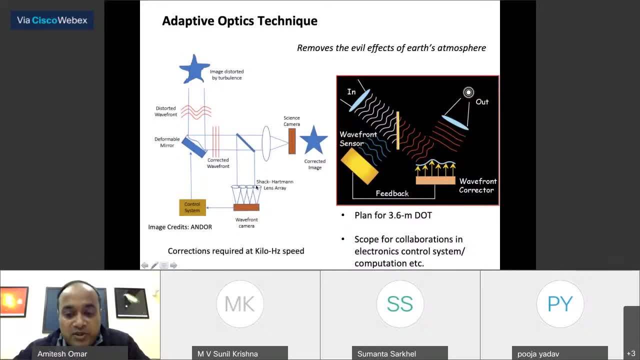 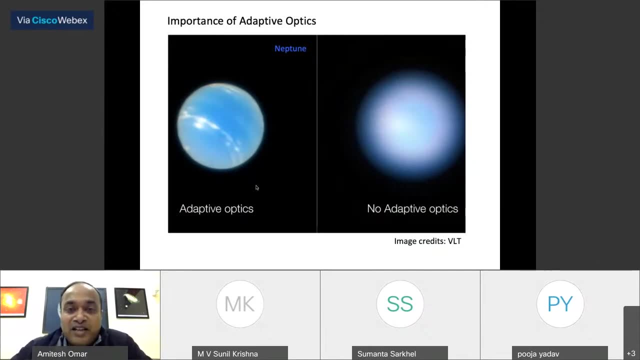 the wavefront sensing and controlling the mirror. so there is a lot of scope for electronic control system and computation here and that will be really one thing to pursue for 3.6 meter telescope in the future. and what you see is the importance of adaptive optics. this is an image from one of the largest 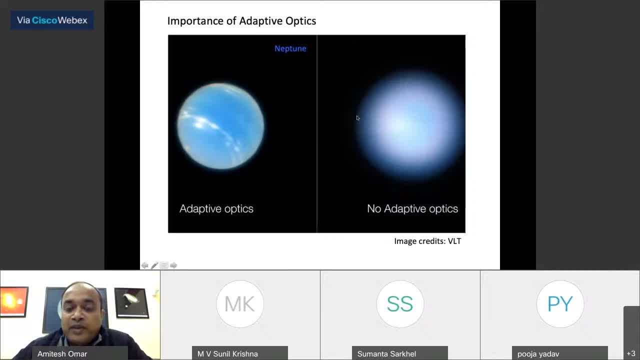 telescopes called VLT, where you see, when there is no adaptive optics, this is what atmosphere, earth atmosphere does to the images. and when you switch on the adaptive optics technique, you see the sharp image. this is the image of Neptune, and so adaptive optics does a wonderful job, in fact, at 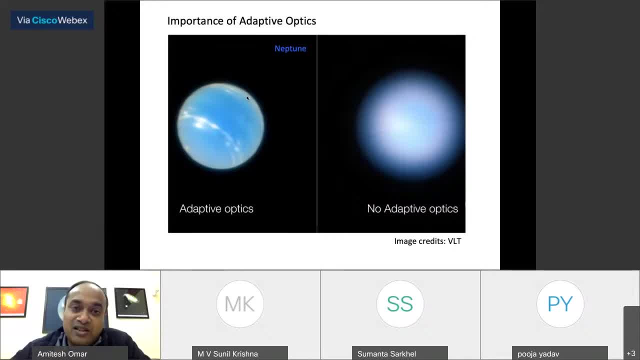 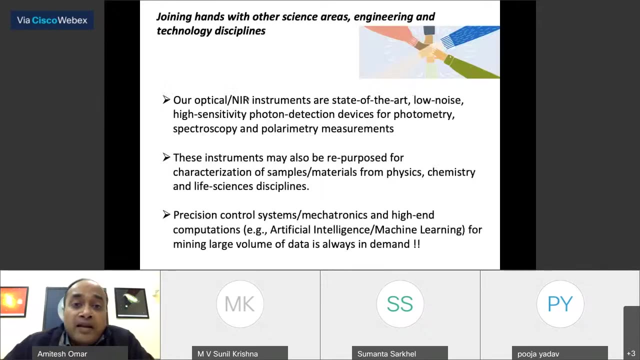 the ground-based telescope. you know it just, any large telescope now, like four meter class telescope, has to have it up to optics. this just cannot, you know, go without that. so we have to build such an adaptive optics, you know, instrument for our telescopes, just to you know, bring out a very 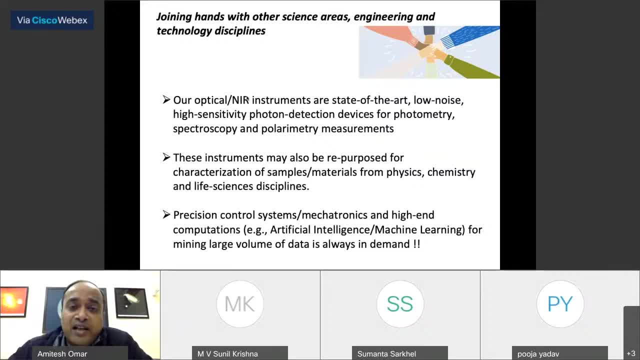 precise points about what can be the collaboration area. collaborating area so our optical and IR instruments, which we have. of course we put it on the telescope, but sometimes they are not on the telescope, they are sitting on the ground and they are state-of-the-art. they have a very low noise because we 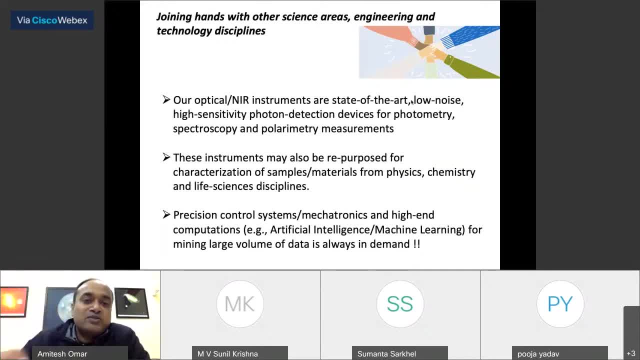 are detecting one photon per second, so our noise has to much lower than that electronic noise present in the system. they are really high sensitivity. you know devices we can do- photometry, spectroscopy and polarimetry- and there has been a discussion on whether these instruments can also be repurposed for 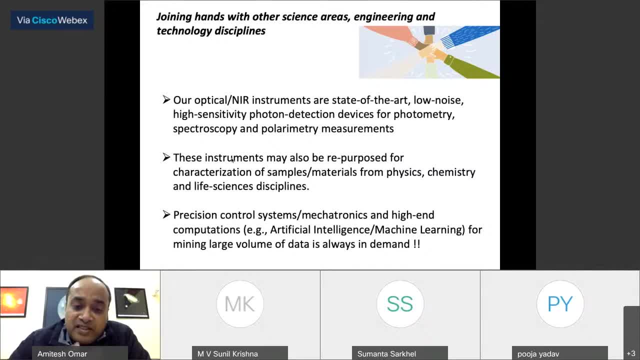 characterization of samples or materials from, let's say, the physics labs- chemistry, you know whatever it can come- are as well as the life sciences, because we know that some of the similar instruments are employed in such laboratories. of course, our instruments are much bigger and much more, you know. 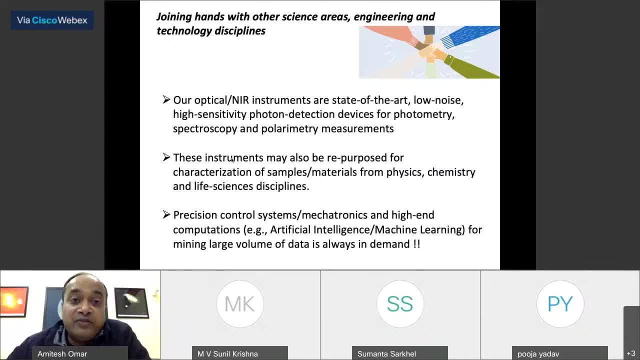 sensitive and so whether they can be repurposed, and that is one area definitely to explore and join hands in. that. and another area which is really very important and we are always looking for that is a precision control system. all this telescope, all these techniques require a very precision control system and very 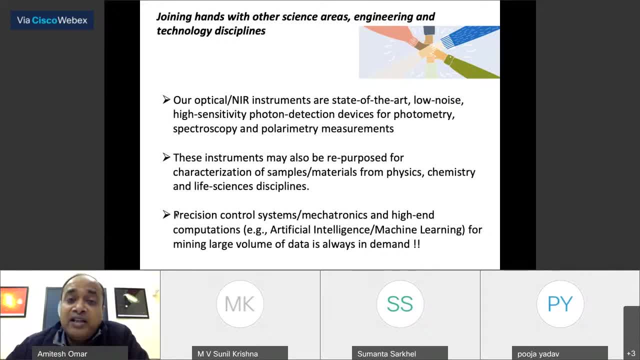 precision mechatronics and high-end computations, particularly if you talk about artificial intelligence and machine learning, because we actually collect large volume of data and it's not possible for humans to see the data by eyes and you know, and a lot of the data that we collect is not possible for humans to see the data by. 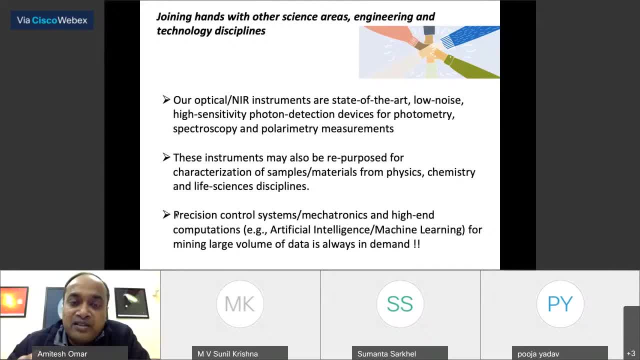 eyes and you know, and a lot of the data that we collect is not possible for humans to see the data by eyes and you know, and a life in their lifetime, the data, the data rates are really high now and so we are now looking for the artificial intelligence and machine learning. so 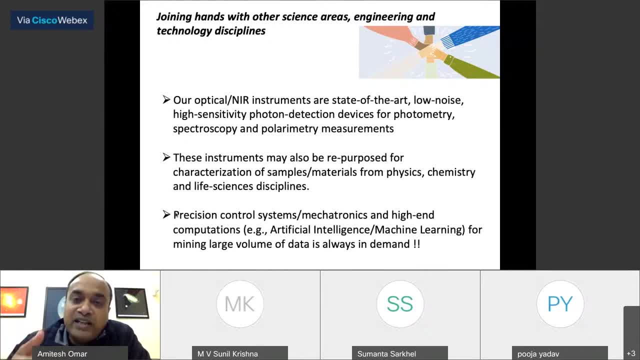 that the DNA analysis can be automated, and there is this. this one area is where astronomy is now looking for. you know people who are, who are already in working in these areas, so this is always in demand. so any student who really makes interest in such things like computation, high-end computation or the mechatronics- 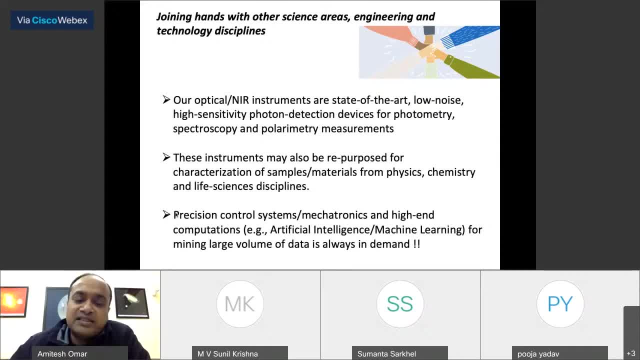 And mechatronics can be very simple things like making robots also, and that's something we also do- a very similar kind of thing, I mean telescopes- can be considered as a very precise, you know, the robots which have been trained to do a very specific job. 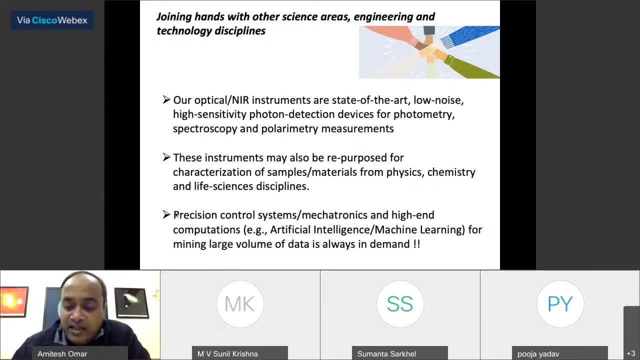 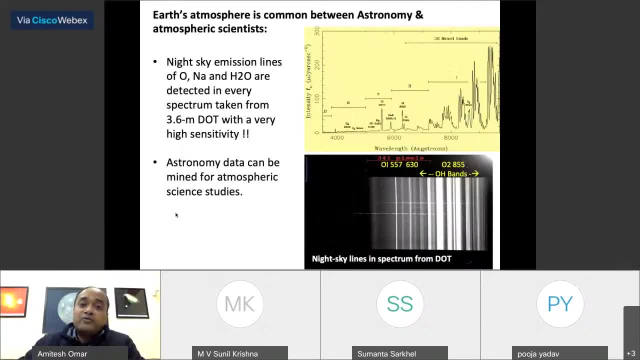 And so these are some of the areas where we definitely like to collaborate so that our telescope systems can be improved in future, And one of really. I just point out that, if we just talk about the science now, I understand that there is a lot of interest in the atmospheric scientists to look at the atmospheric lines. 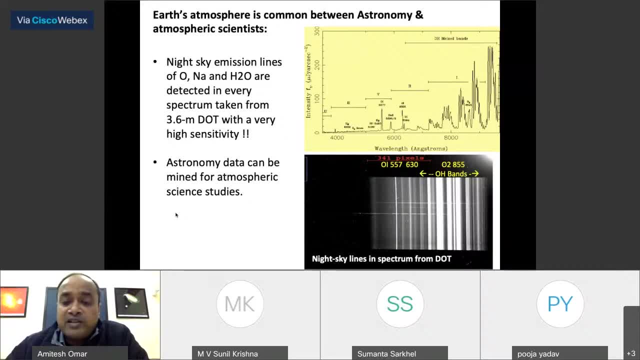 emission lines And in fact, I just point out that every spectrum we take from 3.6-meter telescope actually has this information. It has very, very high sensitivity. So, particularly if you look at this spectrum, what we are interested in? this faint structure. 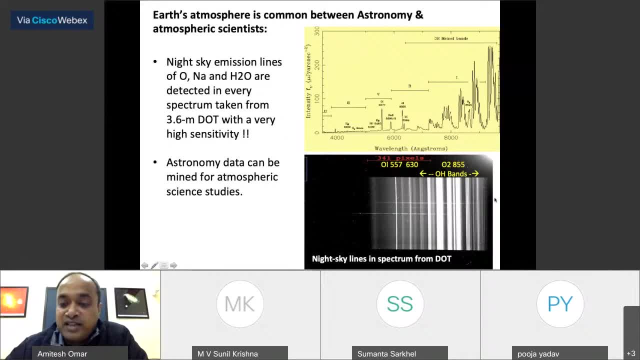 line. what you see, This is actually the spectrum going from blue side to the red side, And this is our interest, and rest is dominated by atmospheric emission, Earth's atmospheric emission, These typical lines like 557, 638.. I mean, if you talk to atmospheric scientists, they really do this kind of work. 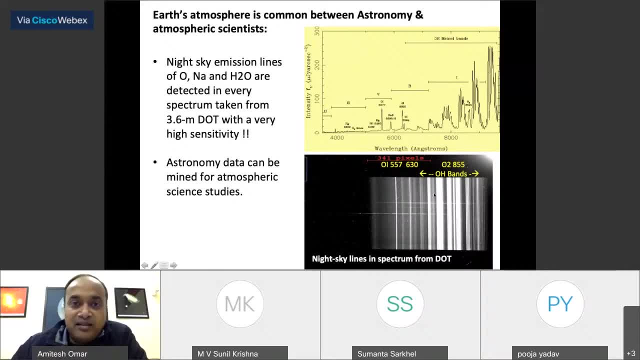 And this is something there in data, in every frame, every you know image we take. it is there in our data and we have to throw it out because that's a nuisance for us, But this is a data for, you know, many atmospheric scientists. 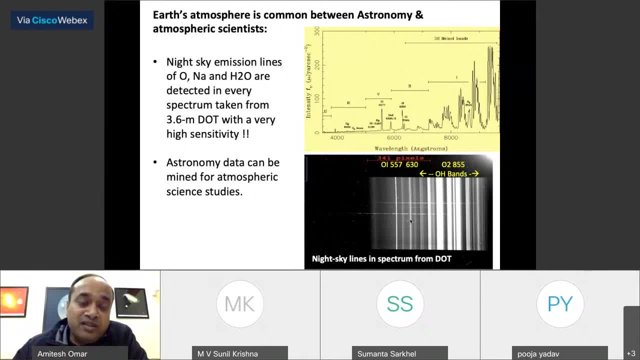 And some of the I know, some of the you know- institutes, astronomy institutes, do such kind of work in collaboration with atmospheric scientists, And so there is a scope for data mining also. All this data which becomes, you know, publicly available after a certain period, can be mined. 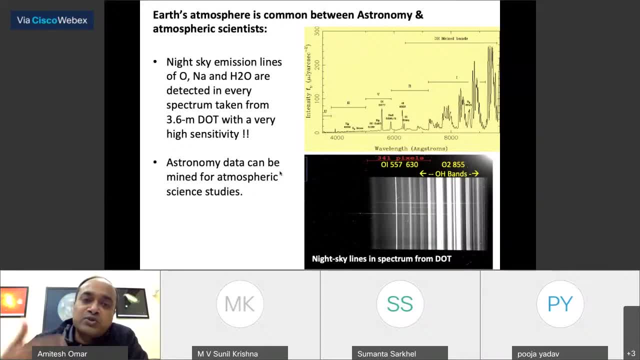 for atmospheric science studies, or it can also be repurposed to do the atmospheric science studies as well as the astronomy. you know it's like it can go on together also, And so I really, you know, appreciate that such programs should be taken up. 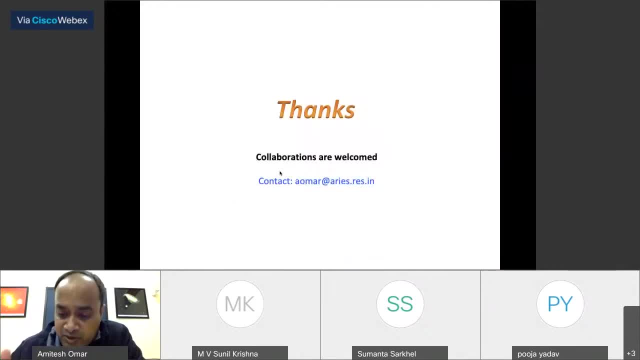 And so, Yeah, So that's. I think that that brings me to the end of this talk and I will be, you know, happy to take questions and comments, And I particularly emphasize that we are doing all kinds of collaboration and people can. 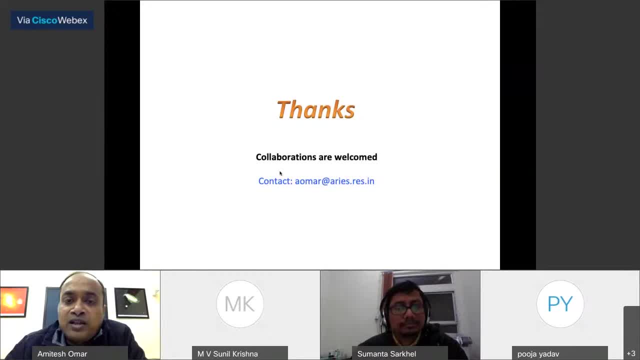 contact us- That's my email- and my colleagues also there. you can find their research interests from the website. So thank you very much. Okay, so we can accommodate a few questions now. So the first question is: if all the stars are in the sky, what would you do? 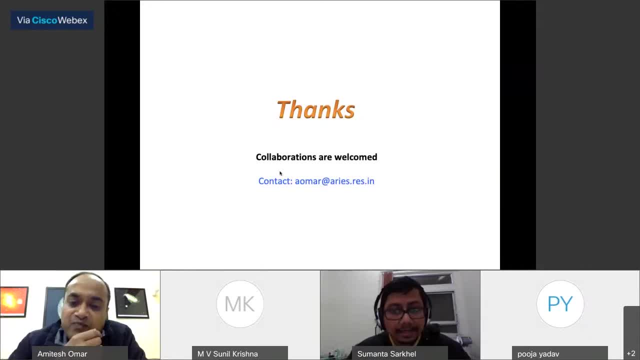 So the first question is: if all the stars are in the sky, what would you do? Okay, So the first question is: if all the stars are in the sky, what would you do? So the first question is: if all the stars are in the sky, what would you do? If all the stars collapse, at the end is the universe is dying, basically, Eventually. you know stars. of course, this is going to take a very long time. What is the question is that it's just theoretically. that's true. 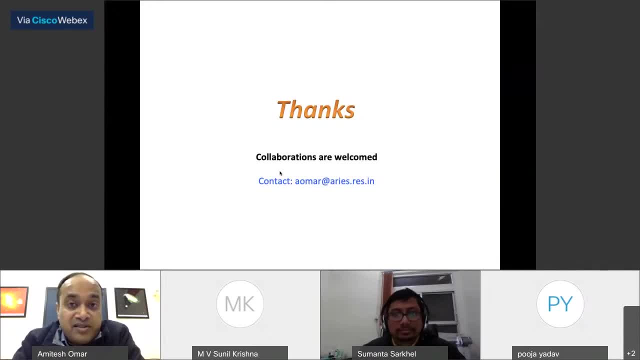 At the end, the universe has to become dark because there will be no stars. But that's far, far away. Okay, Okay, Okay. the next question is: how does the deformable mirror responses so fast while correcting the wavefronts? 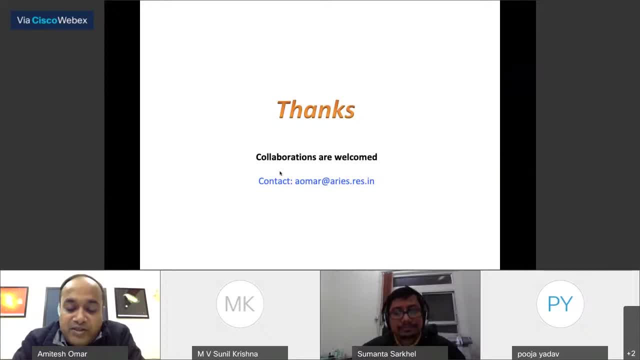 What are the computational challenges here? Yeah, so actually the computational challenges are: first thing is the latency. you cannot have latency in the system, So one has to sense the different, calculate it and send the command so that this happens in a period shorter than the atmospheric. 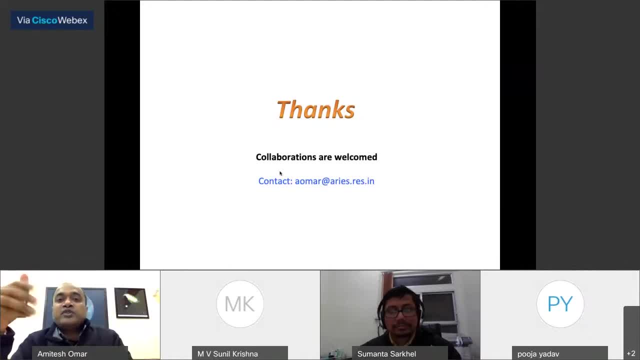 Okay, So you know time scale changes. So it actually the atmospheric time scale changes every millisecond level. So what has to do this computation? apply the correction faster than that And so that the correction which we are applying is valid, because after a few milliseconds, 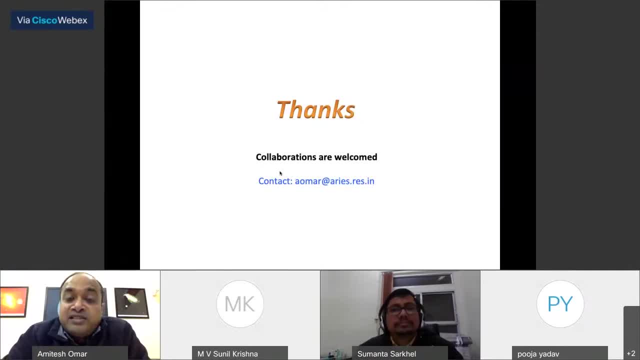 that correction will not be well, And so that is the main challenge: is the fast computation and create computation. what should be the algorithm? because, finally, the wavefront sensing will not be happening at infinite resolution. this will happen at a certain resolution and then we have to interpolate. 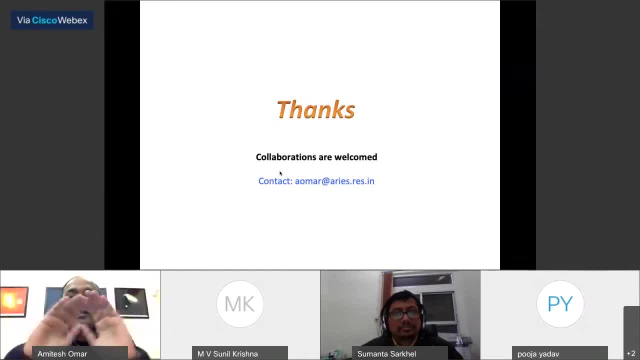 or extrapolate the data So that the whole wavefront can be corrected. Okay, So that is the main challenge: the computation as well as the development of right algorithm. Okay, so a couple of questions from my side, And of course there will be other questions as well. 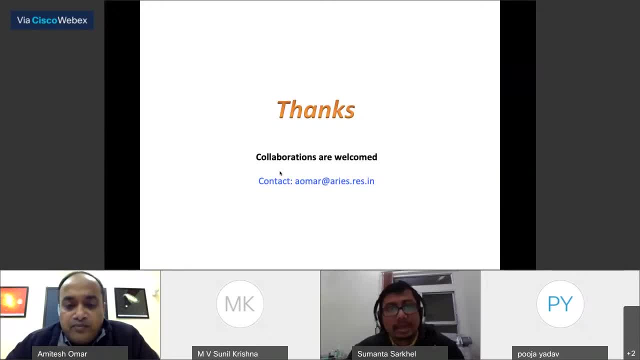 So, for example, what are the like opportunities for our like electronic students or mechanical students or, as a physics students, like they are? all are beating. they're doing like 30 or 40 years, So is there any internship? who can do some projects in this area? development area mostly. 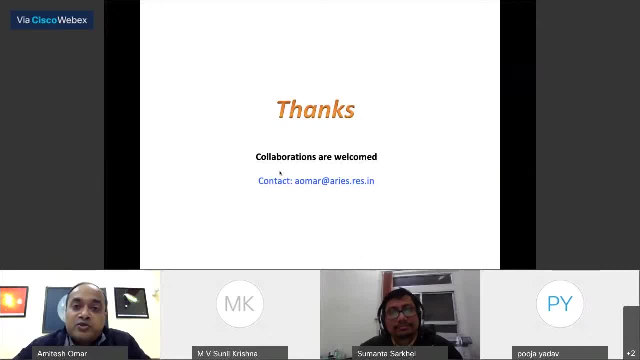 Yeah, I think. I think now there are programs. but even if there is no formal program, that's it. that is something one can develop it. But we are always open if people want to do internship, people want to come for a few. 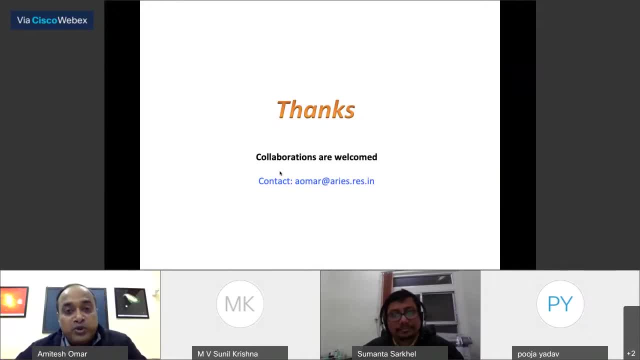 months of project. we can formally do that because we know from universities for science we regularly get students who come here do part of their- you know, degree program, like the project or industrial projects and all that, And so something similar is always possible. you can- I mean they can- contact us and 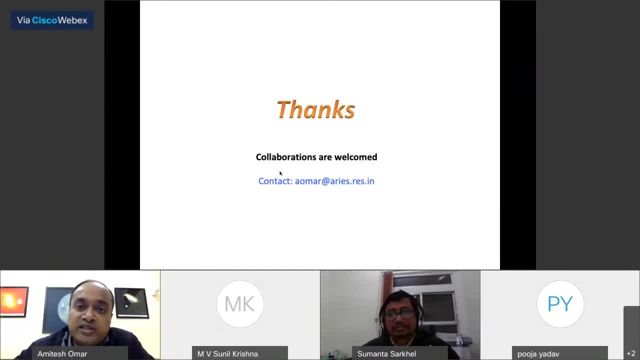 and always suggest some topics to work related to the instrument. Okay, So in either in your spectrograph. so what are the like? spectral resolution: Yeah, so we have varying spectral resolution. we start from about a nanometer, we can go to a few nanometer or we can go to sub nanometer also. 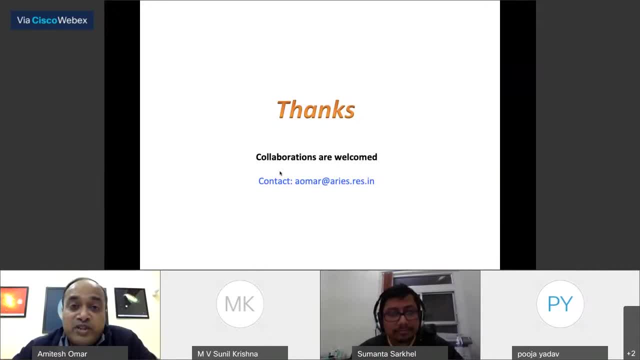 This is what presented. Okay, So essentially we have, of course, in the future we will have a very high resolution spectrograph which will be, you know, like. what we say is something like 0.01 nanometer. 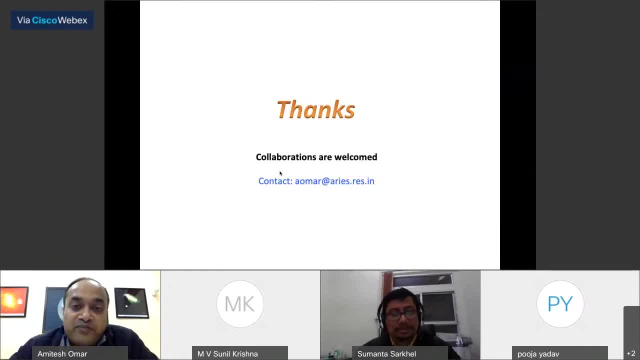 or so. Okay, We have about a nanometer. Okay, There is one more questions. What are the prerequisites for working with like Devastel Optical Telescope as a undergrad, like a short period project, I don't know. I mean, there is no formal prerequisite. 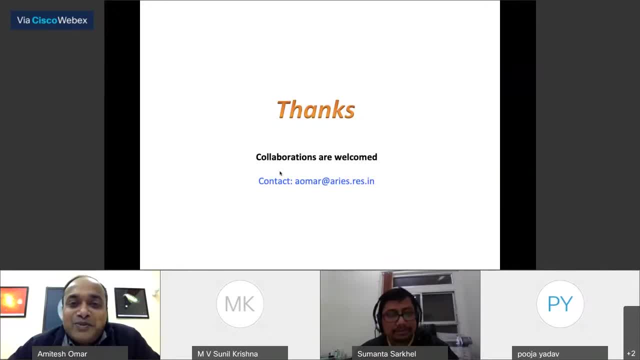 Okay, But everywhere students fit in because it is accommodative. Okay, Okay, Those work, But yeah, but if they are asking for any, like we have a PhD programme, If people want to pursue PhD programme, then they have to have a degree in science history. 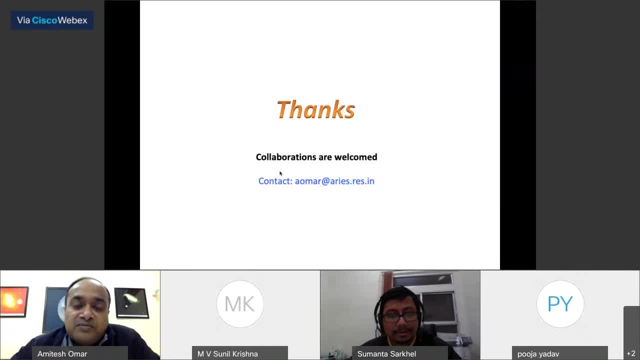 So that is a Master of Science, MSc. Okay, all right. So any students, if you still have some questions, you could raise your hand. so it is there on your right side of your screen. okay, it seems. uh, there is no further questions. 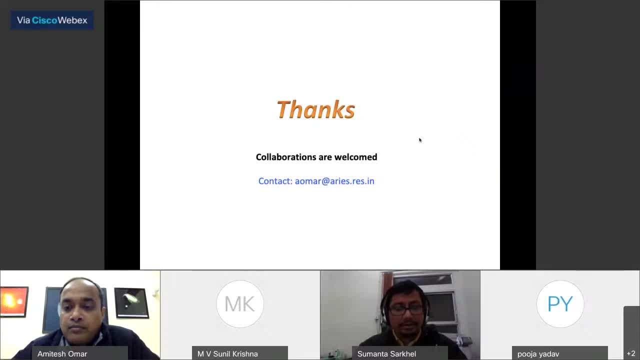 all right. so, on behalf of the organizing team, i take this opportunity to put forward the vote of thanks and acknowledging the support in our finances in this lecture series. so i thank dr amitesh omar for delivering such a wonderful talk. we learned a lot and, of course, our 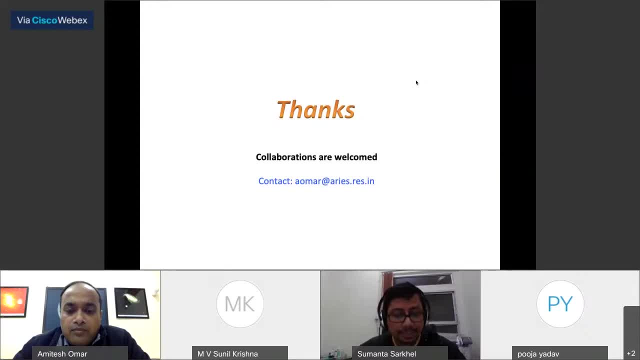 iit students definitely will get benefit in future and i think, thank physics and astronomy club team members, which comes under student technical councils council lighted rookie, for their support in organizing this lecture series. i thank our head of the department, professor gd, and the president of Indian Physics Association, Ruki chapter, and the team members. 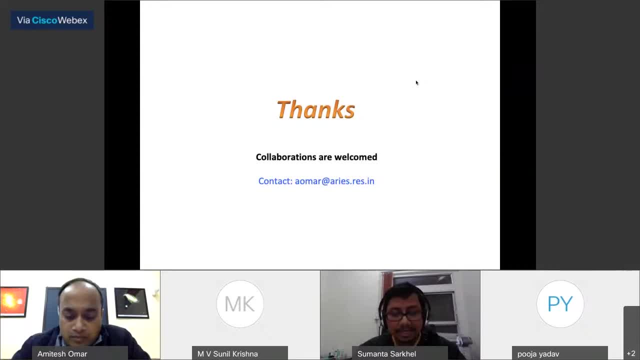 I also thank Professor Anil Gaurashetty for being the instrumental in organizing this lecture series And, at the last, I thank Professor Sunil Krishna and the audience for their attention. Thank you all and good night. Thank you, good night. Thank you.